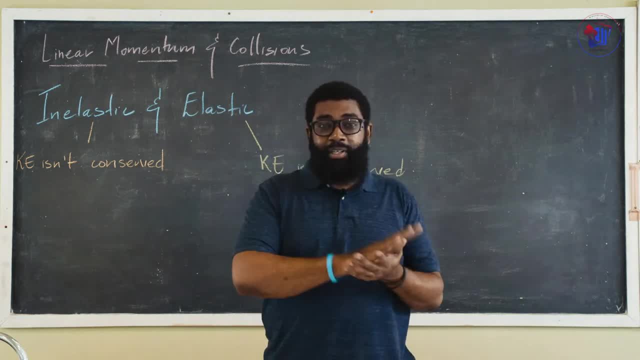 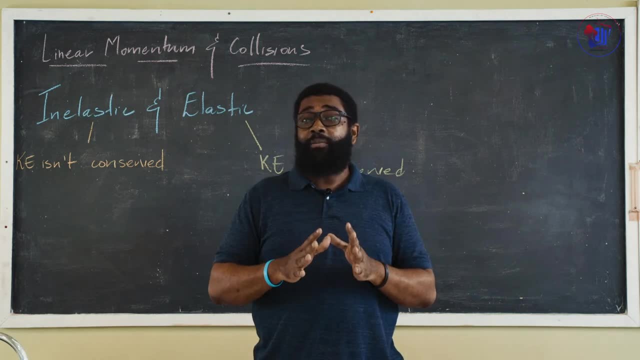 someone was, or you're going to an empty seat and Guyanese do that thing where they hit the seat, Yeah, that's a collision as well. Now, collisions are very, very, very common, Like I said, as long as one object has velocity and it comes into. 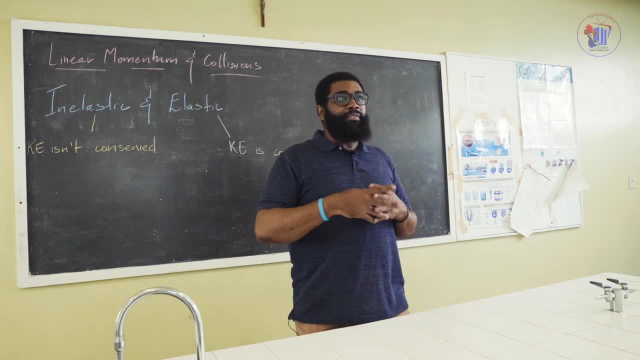 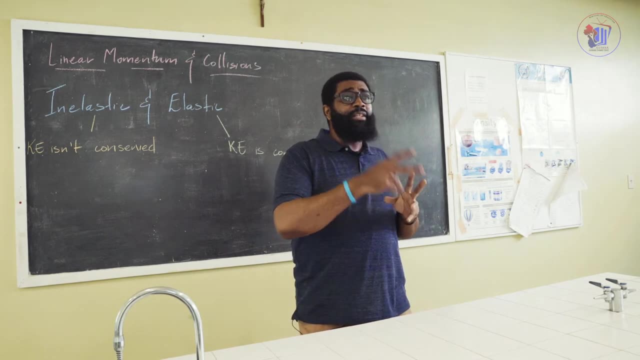 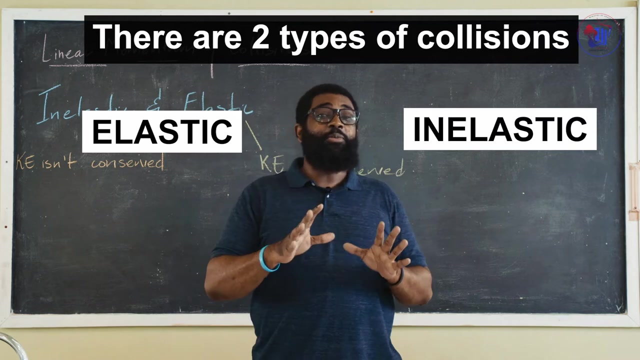 contact with another, it is a collision. The level of violence or severity of the collision depends on the velocities involved. There are two main types of collisions, just two. We have inelastic and we have elastic. Now the cool thing is these collisions are really easy to understand. 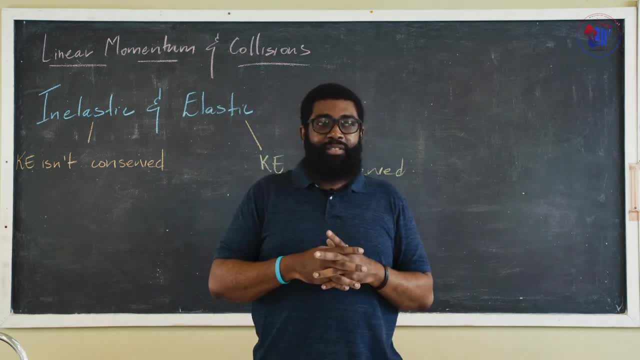 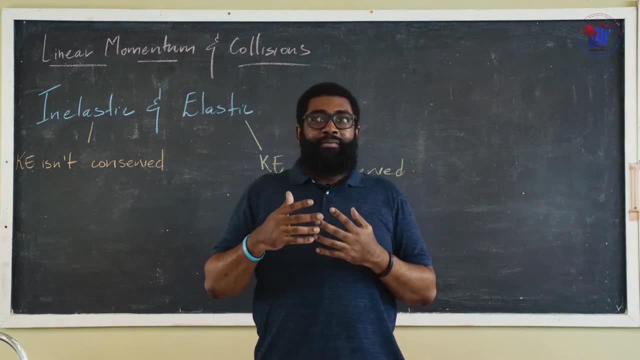 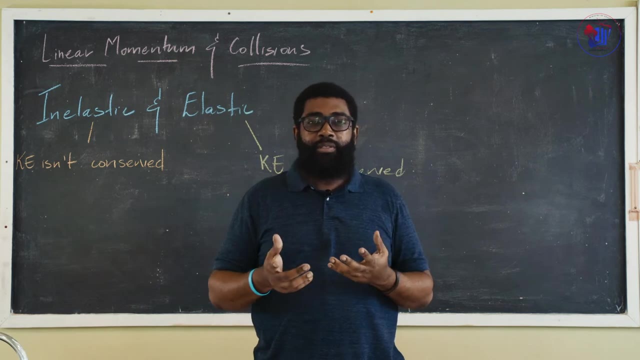 Inelastic collisions are essentially real-world collisions, collisions that happen generally in in in life. um when two objects collide, energy is usually lost. now, this energy is primarily lost as a zone, but there are cases- and it's far more common than you think- where deformation occurs, where the object change shape. 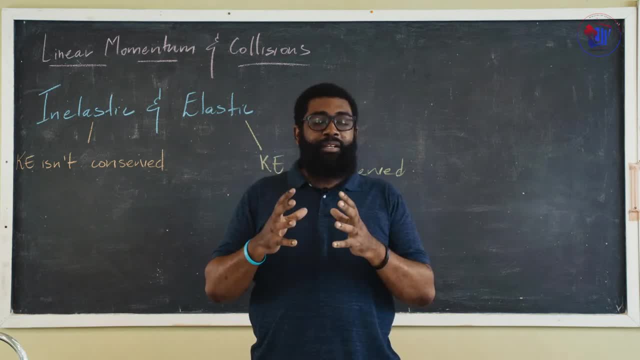 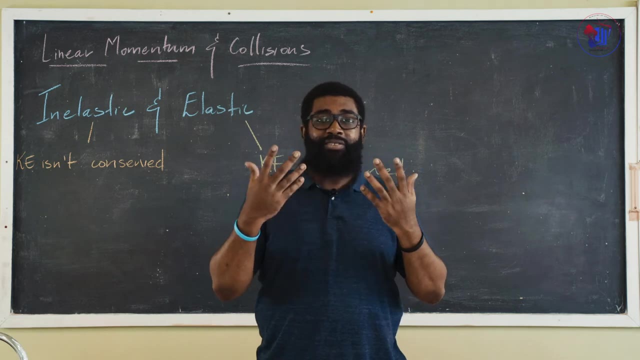 now, um, this causes there to be a more energy before the collision in the entire system and then less energy after. because if, if i do this, this is a very simple collision- i'm clapping and a sound is produced. energy is lost as sound. now there is temporary deformation of my hands. 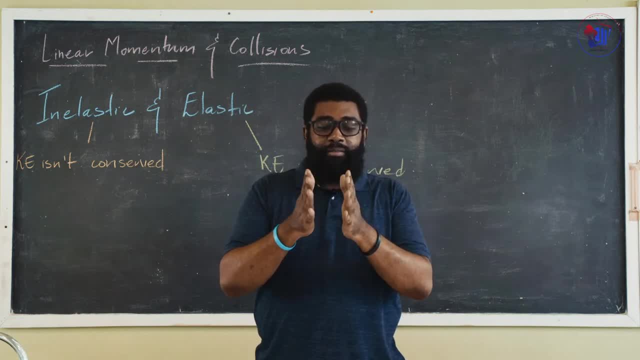 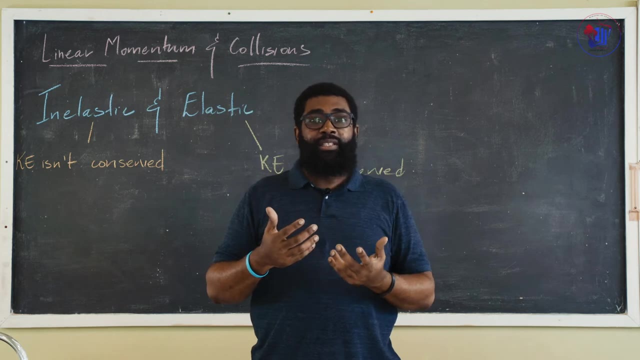 because they kind of press together and that squeezing together of my palms causes them to be deformed temporarily, but it's not a permanent deformation. if, however, a car hits another car or a post, or let's say you drop a um, a metal can, a can of soda, and it hits the ground, that will produce some, or 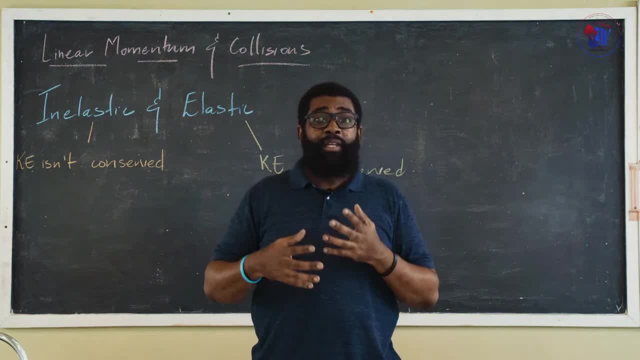 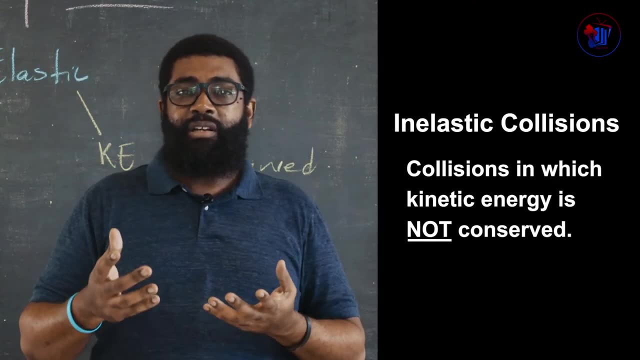 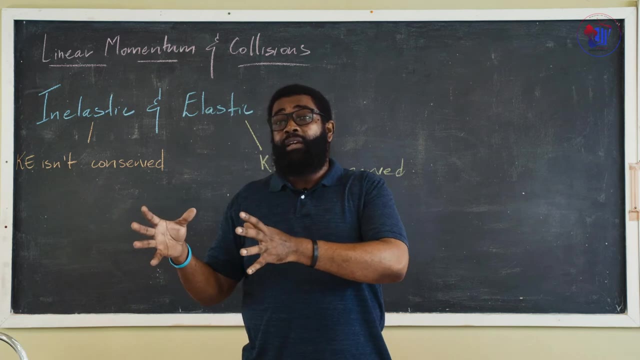 most likely, should produce some form of permanent deformation and energy is lost as a result of these things. so inelastic collisions are simply defined as collisions in which kinetic energy is not conserved. okay, now, there are two important things about every collision: there's the behavior of the objects before they collide, and then there's the behavior of the objects. 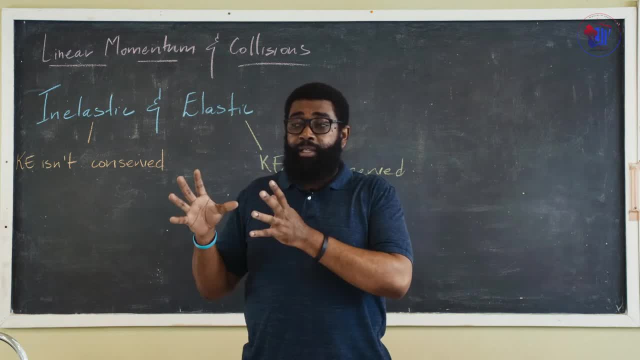 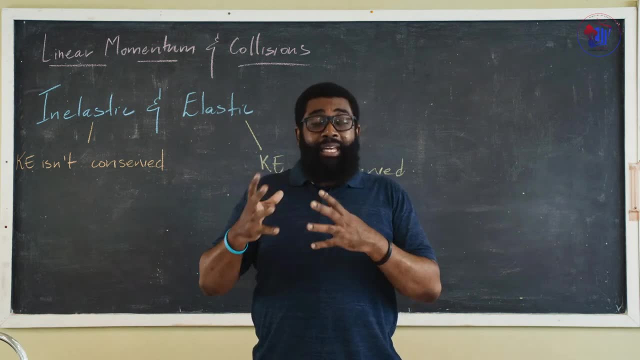 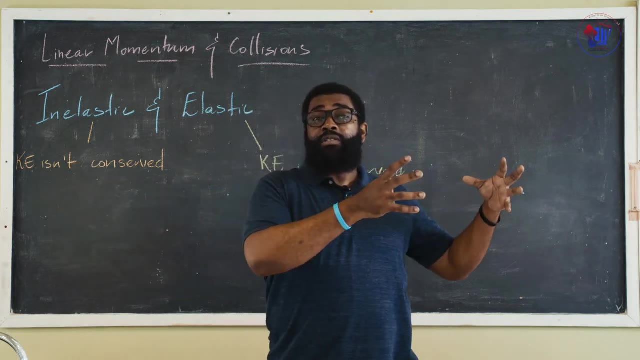 after they collide. before they collide, they have a certain amount of energy and then, after the they collide, they have again a certain amount of energy as well. in inelastic collisions, there is a difference between the total energy of the system before and the total energy of the system. 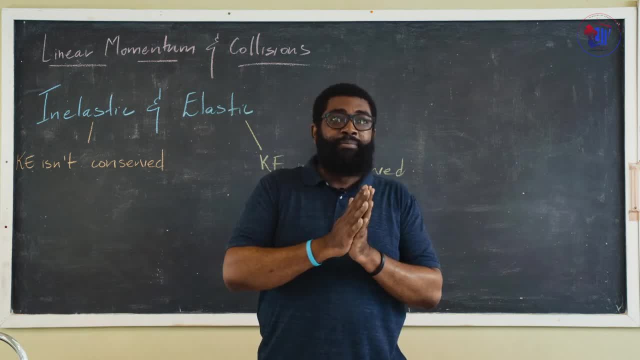 after that collision. so that's how we know they're inelastic. um onto elastic collisions, now elastic collisions i i call them cartoon collisions. um, i've been looking at cartoons all my life. i love them and everybody knows that, no matter what happens in in my personal favorite, 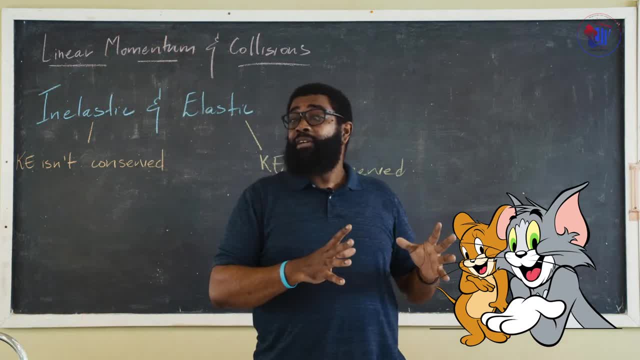 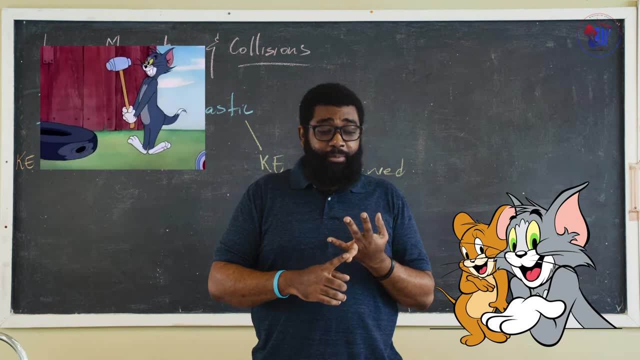 cartoon tom and jerry. no matter what happens to tom or jerry, they go back to how they were before the accident happened. i've seen tom turn into a table. tom has been hit with a hammer. he probably got blown up a few times. but no matter what happens, tom always goes back to how he was. 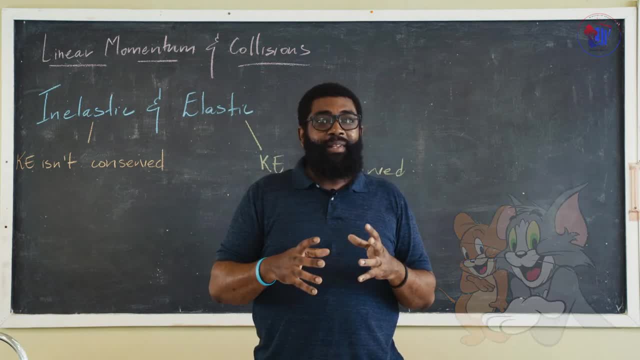 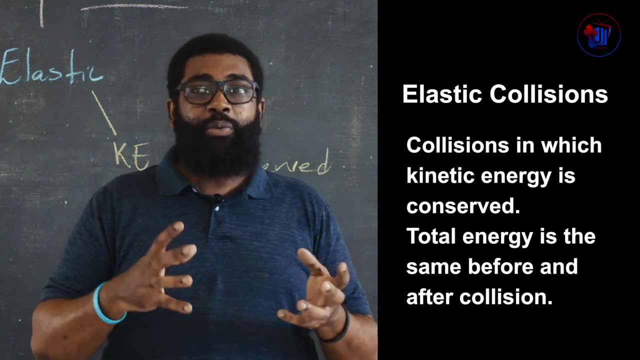 before the collision happened. and that's this. well, i shouldn't say it's close as we come, but that's exactly what happens in the collision scenes. so i don't know a couple clips here that are similar, but an elastic collision. there's really no change to the shape of the object. how? 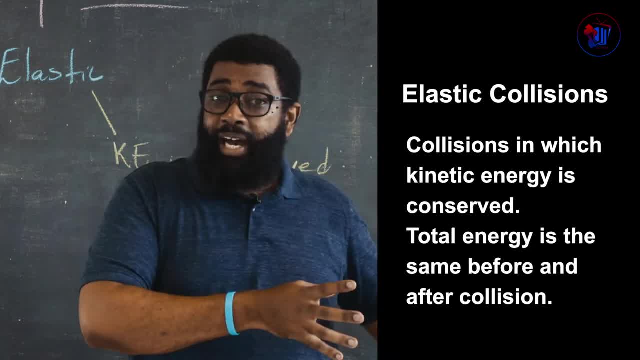 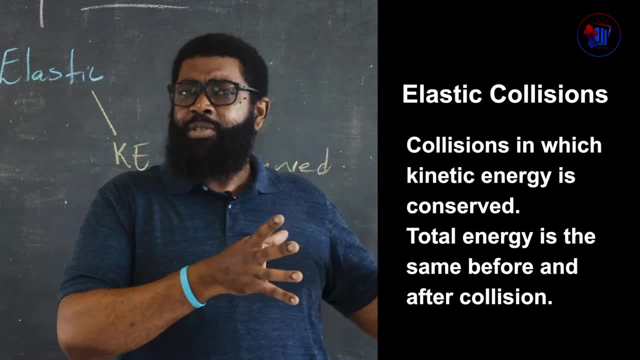 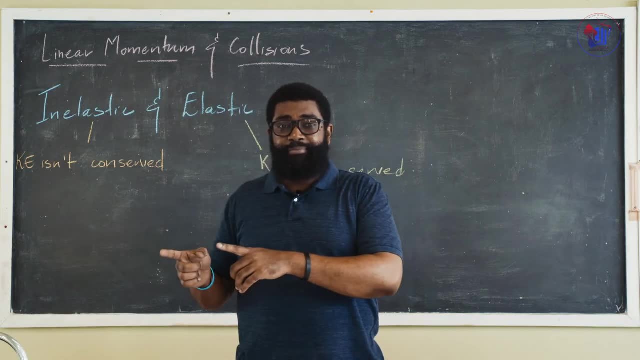 the objects are before they collide is exactly how they are after, and no energy is lost. no kinetic energy is lost. so the total energy before they collide is the same as the total energy after they collide. with elastic collisions. so remember, inelastic energy is lost. these are real-world, practical collisions. 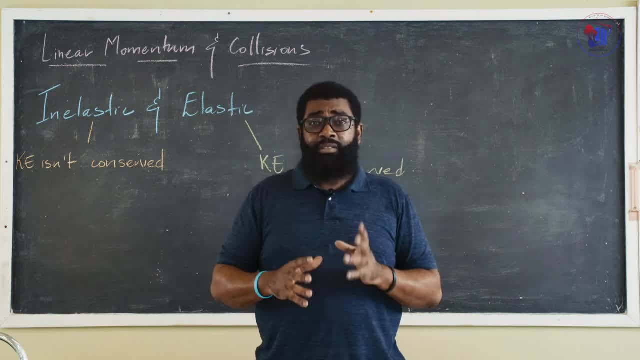 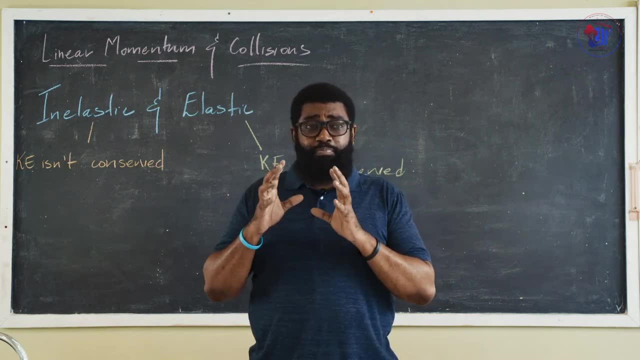 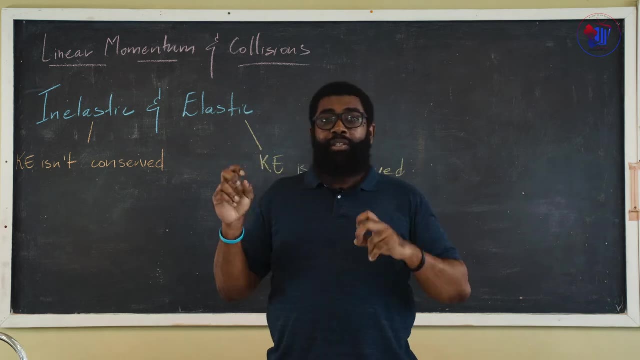 elastic collisions no energy is lost at all. there is no energy lost to sound, there's no energy lost through deformation: the objects essentially remain just as they are now. the best real-world example of an elastic collision is what Guyanese call pools, or, if you're playing billiards, the 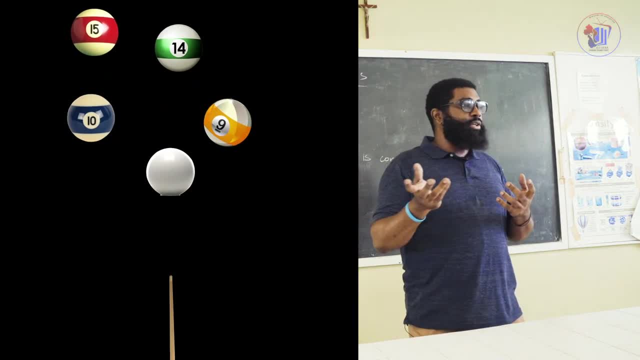 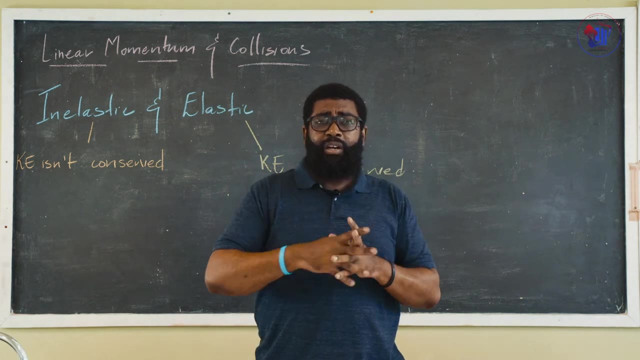 objects don't become deformed. if you hit one pool ball or a billiard ball into the other, it doesn't cause deformation. of course there is sound, but that doesn't cause a tremendous change in the velocity of the objects. also, if you notice, you don't play billiards or pools on a rough. 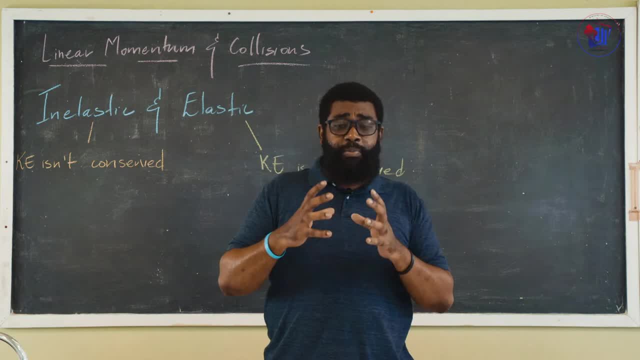 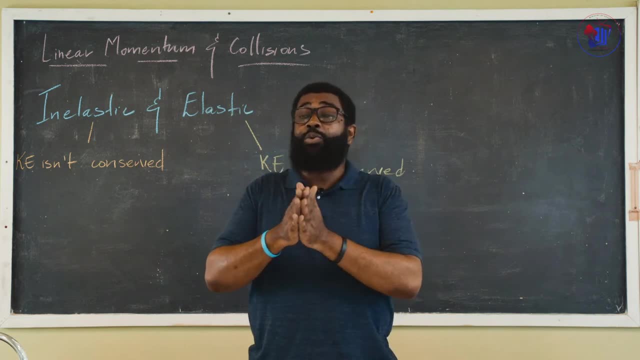 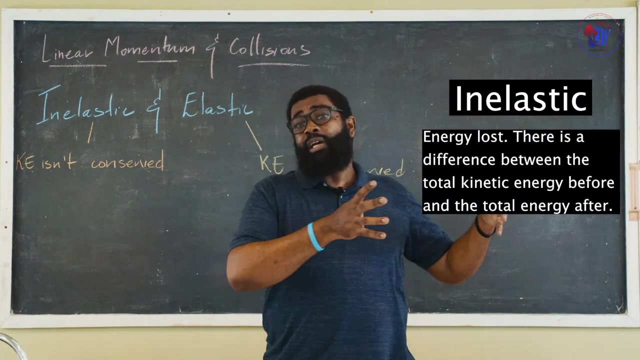 surface. the surface is incredibly smooth. the surface of the balls be incredibly smooth as well, and this is why you can see the collisions are close to, are as close to elastic as possible. so we're capping very, very quickly in elastic energy lost. There's a difference between the total kinetic energy before and the total kinetic 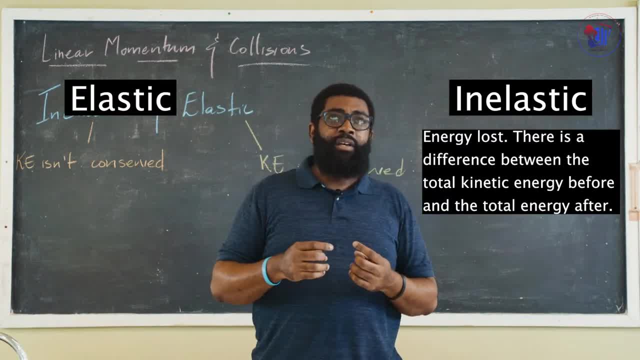 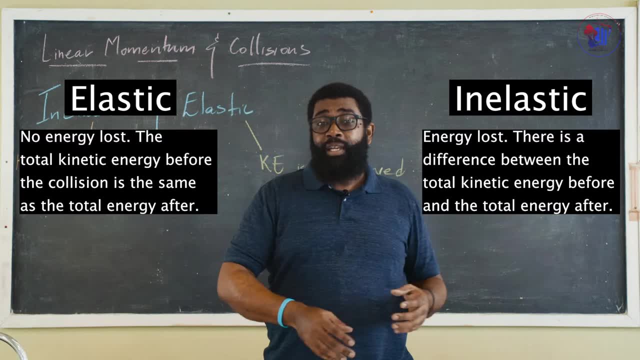 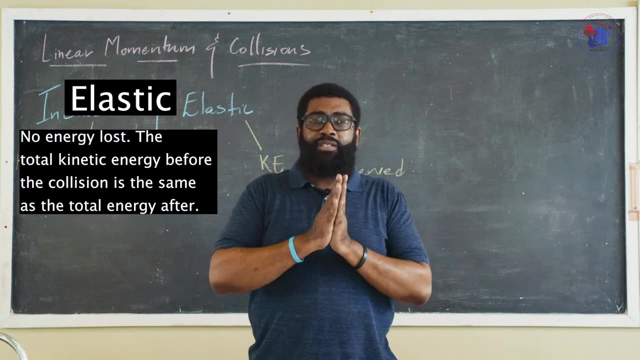 energy after. In elastic collisions, there is no energy lost. The total energy before the collision is the same as the total kinetic energy after. These are the two types of collisions. Now, it would please you to note that we only look at one, We only look at elastic collisions. for 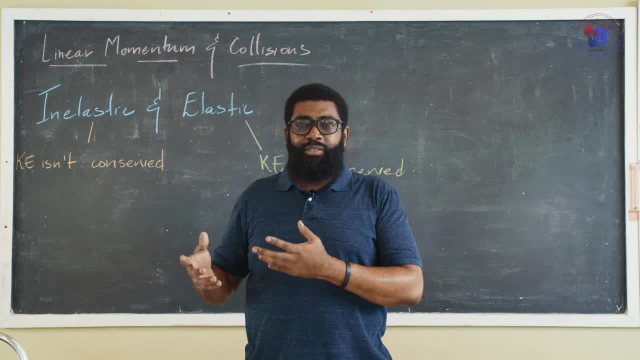 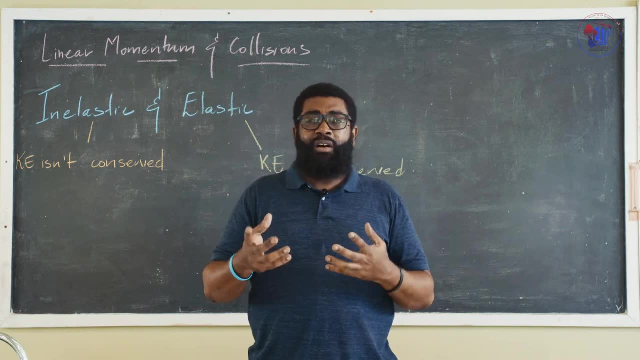 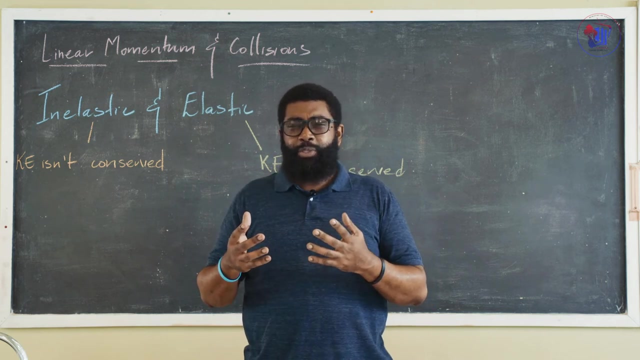 the simple reason that they're easy to analyze. It's easy to assume that no energy is lost. When you go into actually looking at what causes energy loss and how energy is lost, it becomes a bit complicated. For example, if you're looking at, I'm sure you probably see 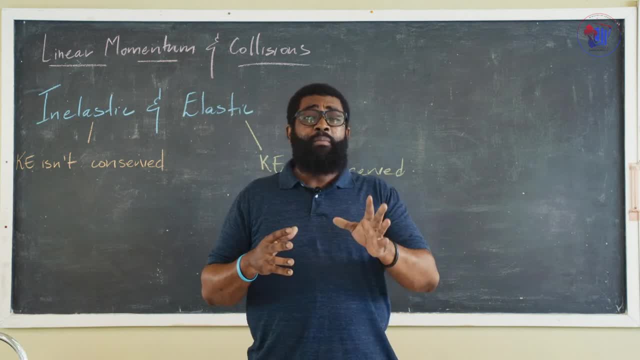 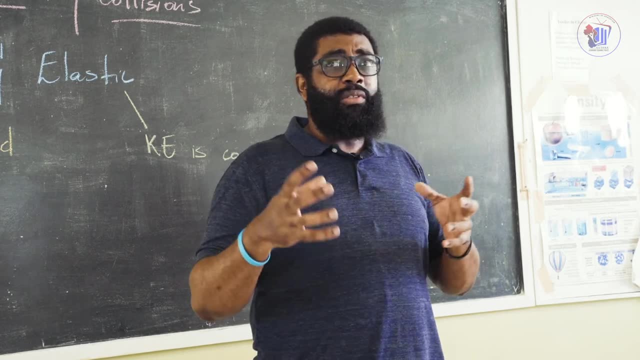 well, actually, no, the advertisements don't come the same, But it was once a point in time when a lot of accidents- sorry, a lot of advertisements- with cars had the whole crash test video and it showed you the car crashing into the wall and they had the crash dummies. 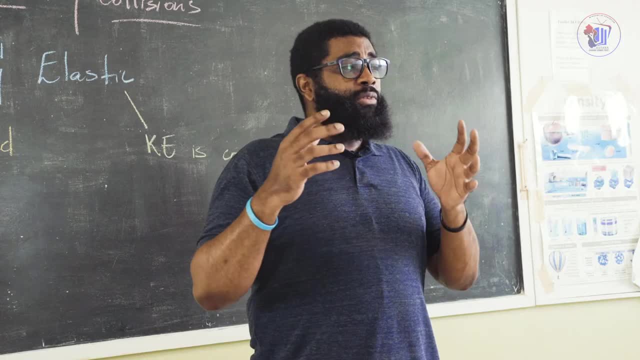 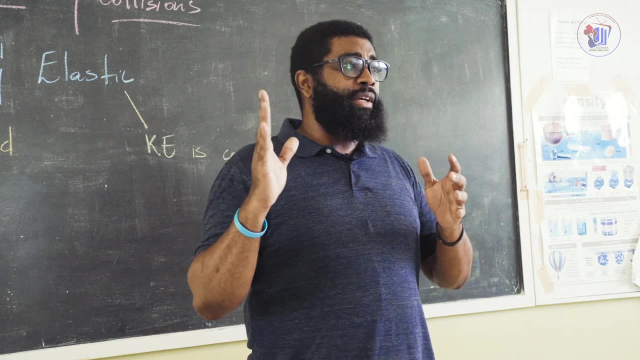 and they showed you how the dummies would move in the car. If you look at a car crashing into a wall, what happens is the essentially the people at the back are moving or start moving a little after the people in front moving forward and the people at 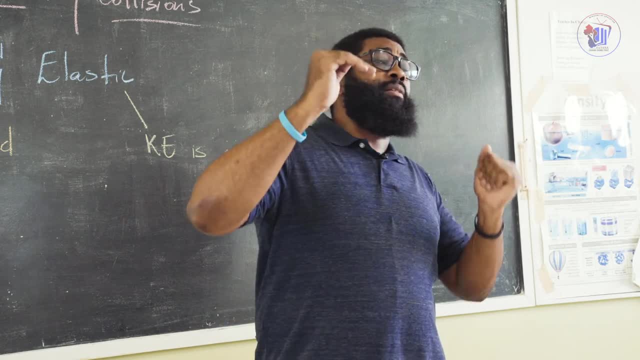 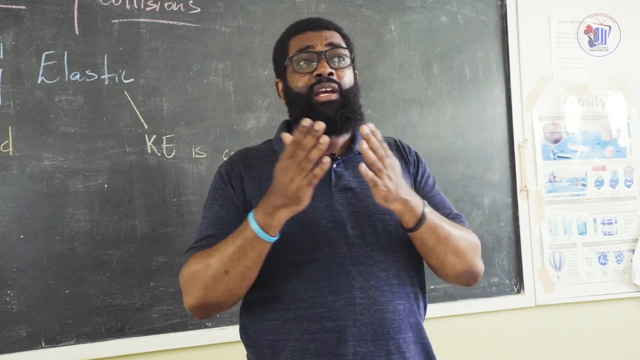 the back come to rest after the people in the front. The back of the car sometimes comes off the ground. All of these little things, all the areas in which energy is lost, would have to be analyzed if we are looking at an inelastic collision. If, however, we're looking at an 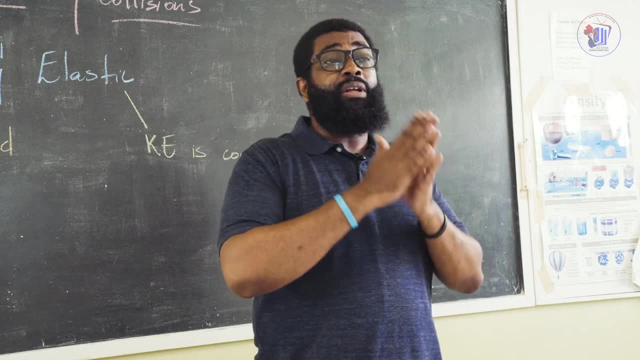 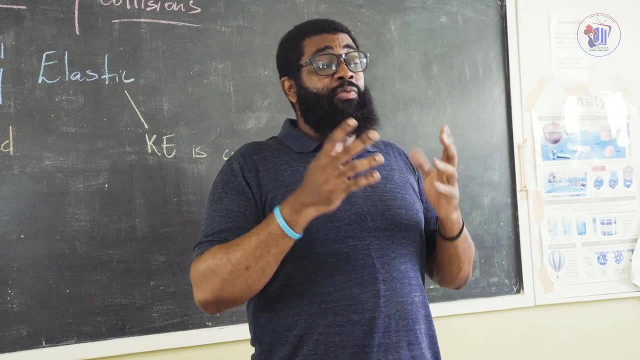 elastic collision, we can just assume that there is no energy lost. We can just assume that there is no energy lost and those things don't need to be considered. So for ease of analysis and for simplicity's sake, for CSEC we only look at elastic collisions. 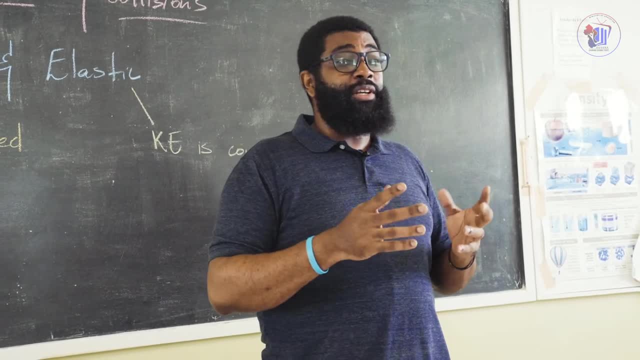 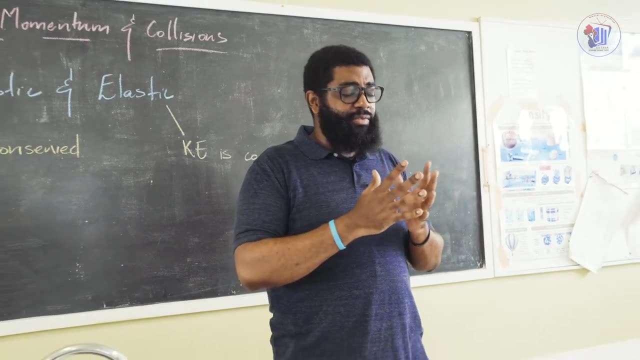 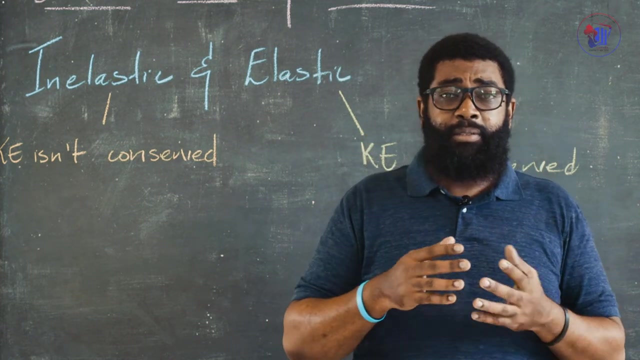 Anyways, it is time for us to do some calculations and some analysis of a few scenarios. But before we do this, the analysis of these scenarios, we have to look at something called the principle of conservation of linear momentum. linear momentum Now. 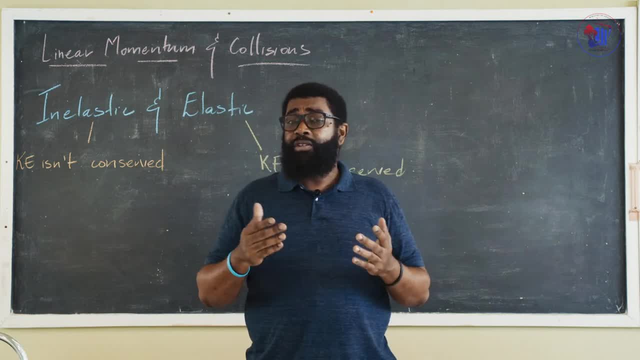 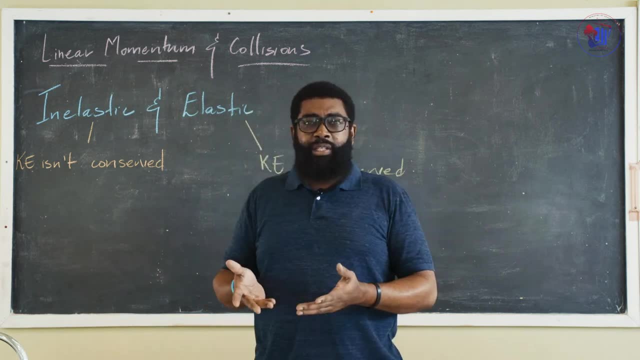 the principle of conservation of linear momentum is that this is something that we can do simultaneously. so what we're going to do now is we're going to look at the principle of conservation of linear momentum. There are different ways to look at this principle. 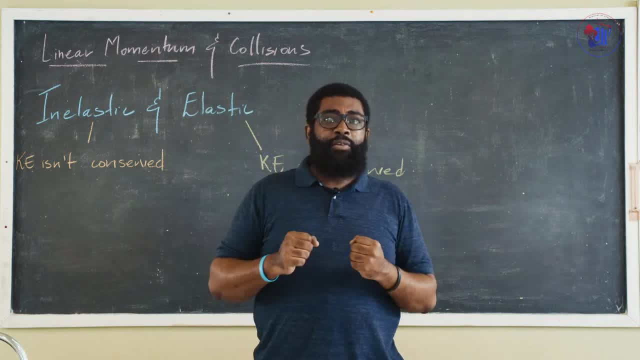 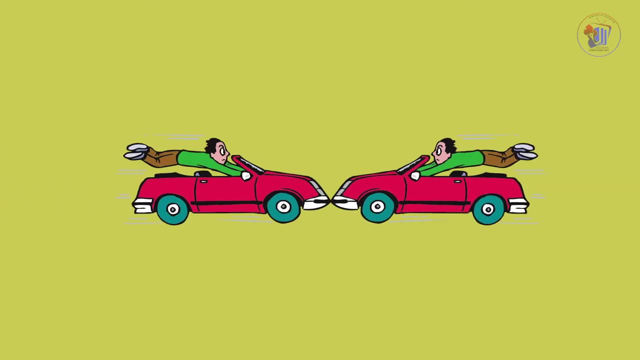 One of them is, for example, the principle of the behaviour of objects. in front of us, We could have two objects head towards you, and that would be one object moving in a straight moving. What happens then? You could have the scenario where you have a slow 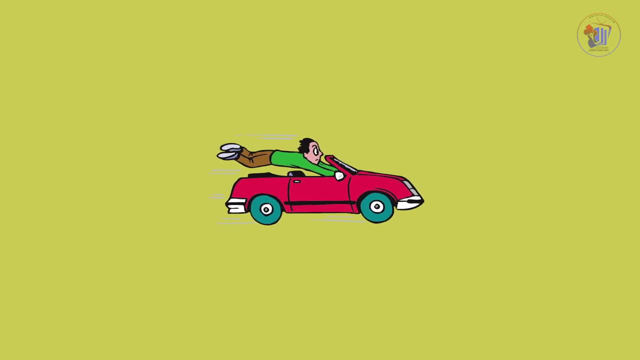 object being pursued by a faster object, The faster object hits the small object and the two essentially combine to form one new object and they move off. You could even have the case of a stationary object being hit by a moving object and the stationary object moves off, while the object that was previously moving. 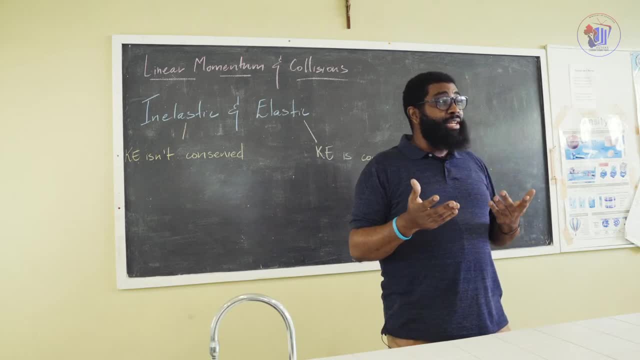 comes to total rest. So many scenarios, and you might be thinking: okay, what do we do with these scenarios? Well, we use something called the principle of conservation of linear momentum. It's a long name, I know very long And it simply 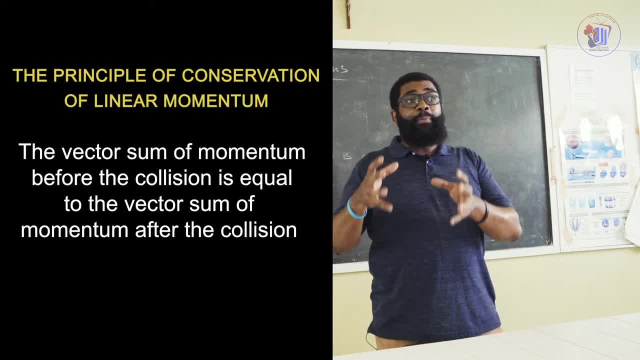 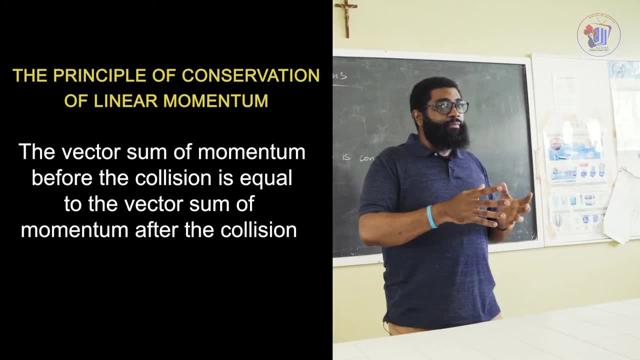 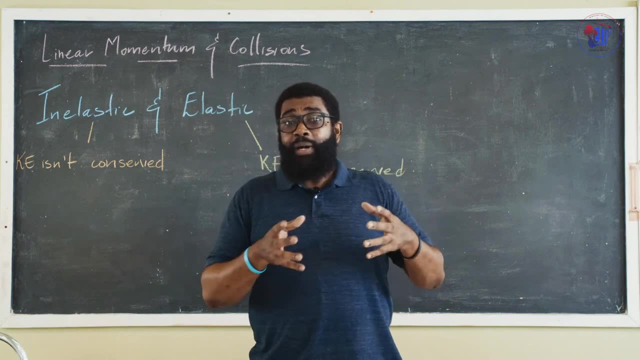 says that the vector sum of momentum before a collision before is equal to the vector sum of momentum after a collision, Meaning if you add up, taking direction into consideration, the total momentum before two objects collide and then you add up the total. 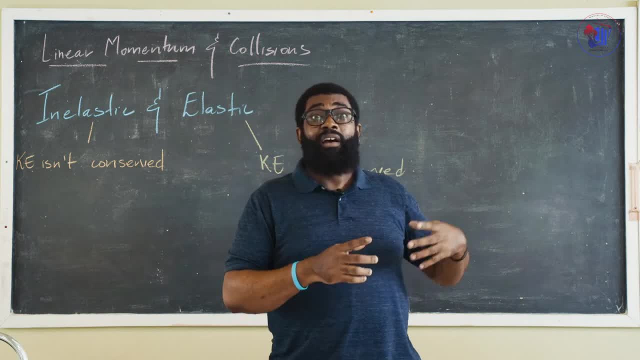 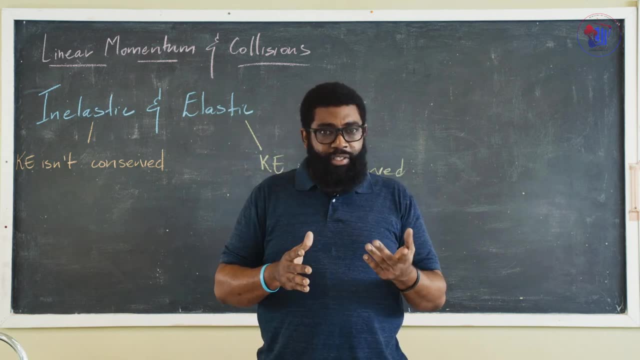 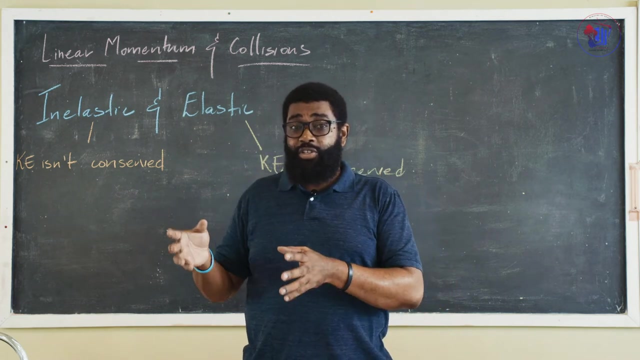 momentum of these two objects, with direction considered after they collide. By this principle, these two values should be the same. There is a condition. The condition is that the collision be elastic, That is, kinetic energy is conserved. If this condition is not met, or it's not assumed, then the principle 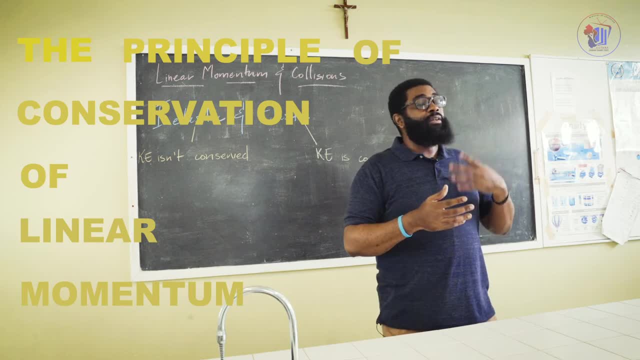 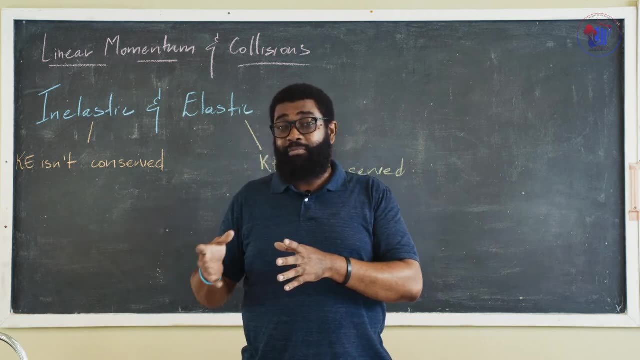 of conservation of linear momentum- that's an example of a linear momentum- is equal to the vector sum of momentum after a collision. Such a long name does not apply, So let me go over it again one more time. The vector sum of momentum before a collision- meaning you take direction into consideration- is 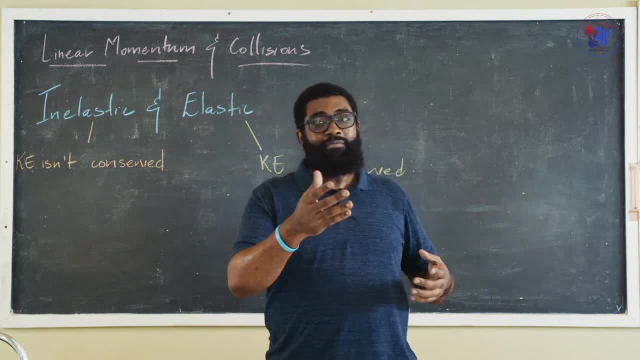 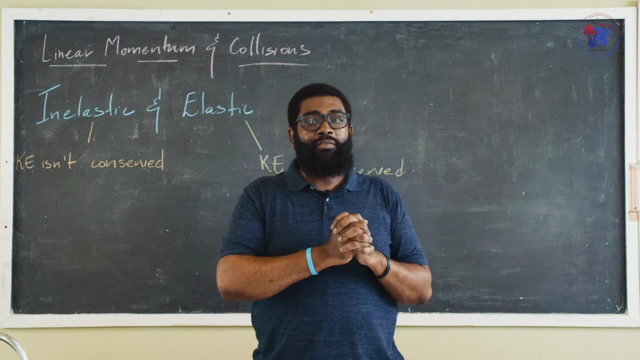 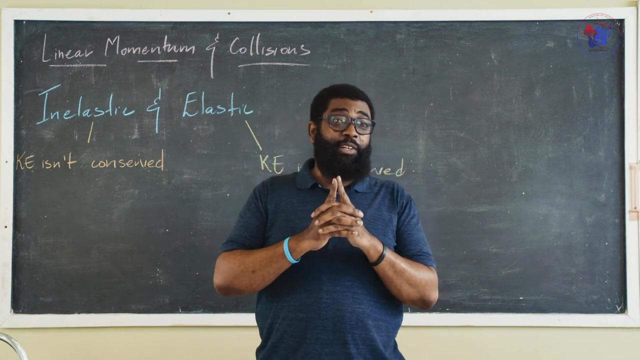 equal to the vector sum of momentum after a collision. again, direction is considered as long as the collision is elastic. That is the principle of conservation of linear momentum. It's time for us to get some examples. Grab a pen, paper, your calculator follow. 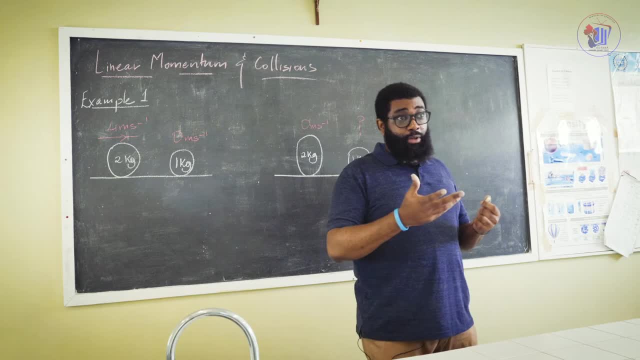 along. Welcome back. I hope you enjoyed this video. If you did, please subscribe to the channel. I'll see you in the next one. Bye, I hope you have your books, pencils or pens and your calculators, because we have a nice. 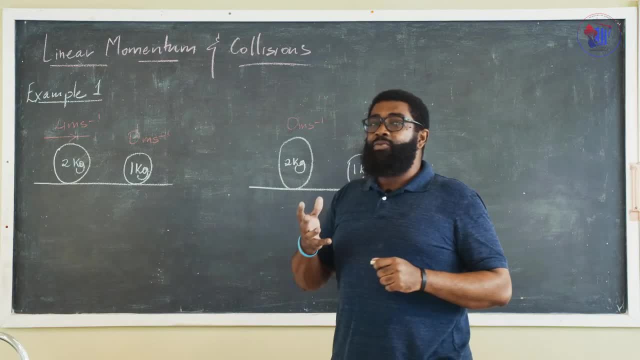 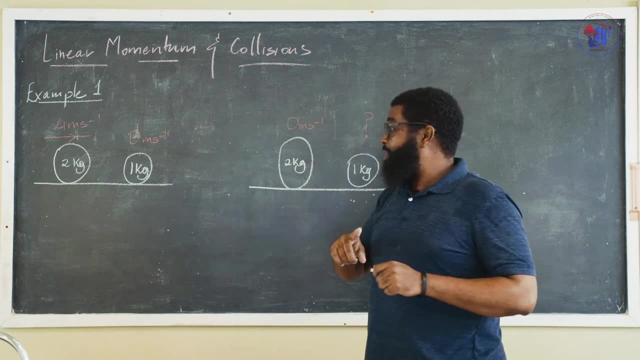 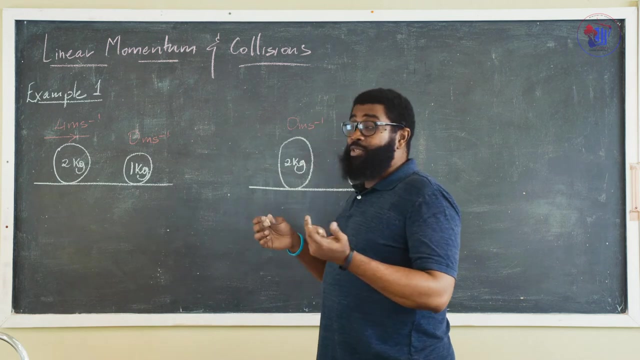 little example to look at Now. I use spheres to represent my masses because they're easy to draw. I'm not going to draw any stickmen for you folks to laugh at my stickmen. I indicate my velocities with numbers and arrows for direction. The directions be very, very important. 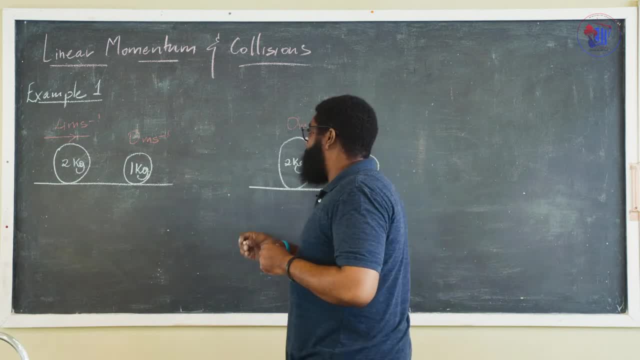 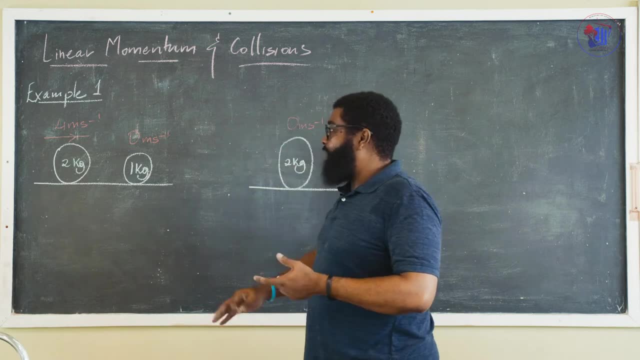 Do not pay attention to the thought. Now let's also summarize some of the principles of conservation of linear momentum. There are some principles that I will give you in a short while. You can use the exercises I already talked about. That's the transportation. 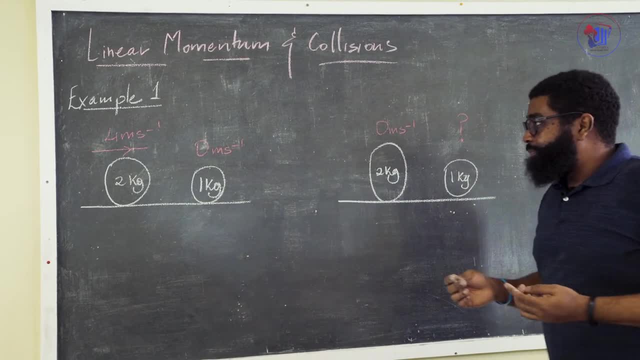 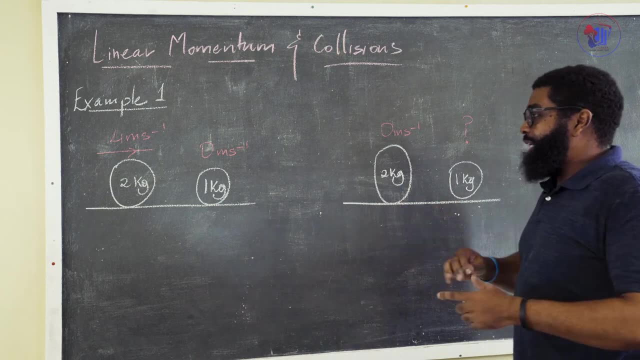 principle And the other principle. I'll give you the demonstration of how to use it in the next lecture. I'll just do a quick demonstration of how I use the example. We have example 1 here, And I must add that this is how the system- and by system I mean the masses and the objects- involved behave before collision and then this is how they behave after. Before and after. before and after Now. by the principle of conservation of linear momentum. by this principle, if this collision is assumed to be elastic, the vector sum of momentum here will be elastic. 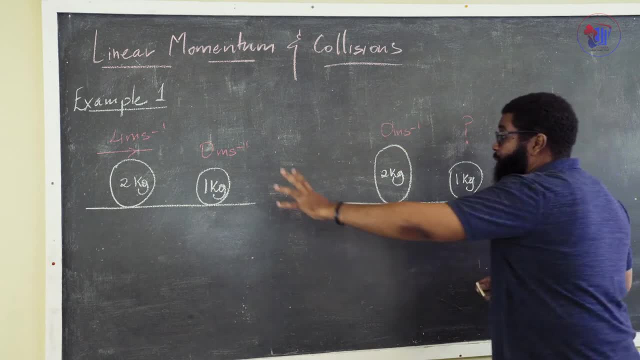 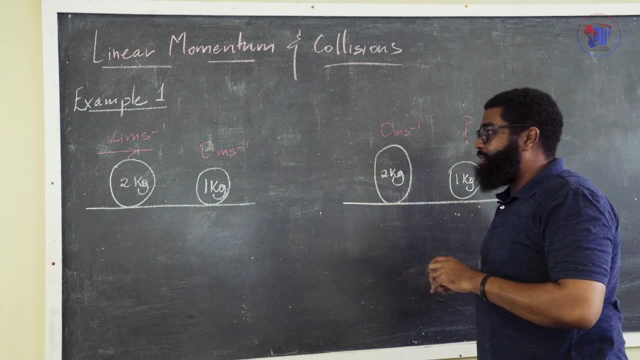 And I'll move on to the next one. the vector sum of momentum after a collision, which is the performance here, is the same as the vector sum of momentum here, meaning whatever is the total momentum over there should be the same as the total momentum over here. so just let me get you used to how i 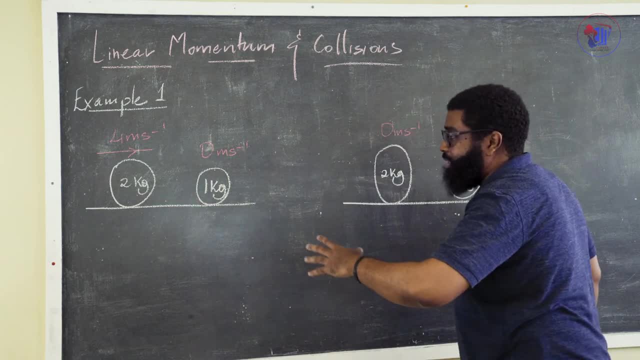 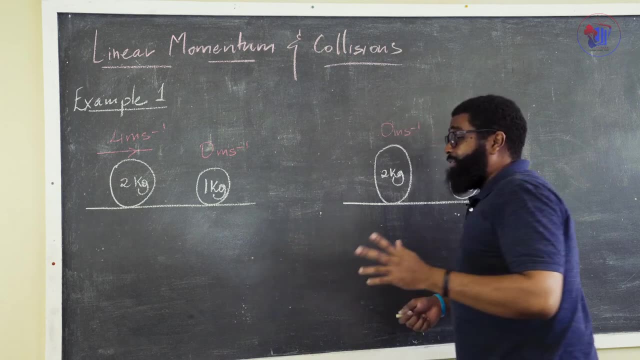 indicate things. the masses are indicated in the spheres and the velocities and their directions are indicated above, if you notice, zero meters per second. now i don't need to give a direction to zero meters per second, because zero implies it's stationary, it's not moving over. here we have. 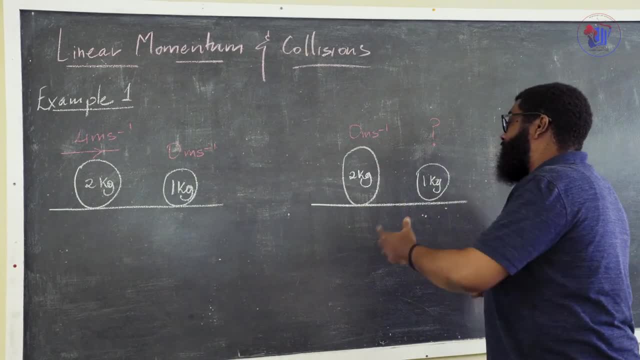 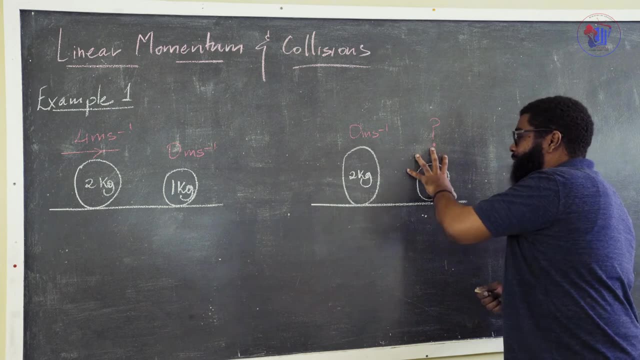 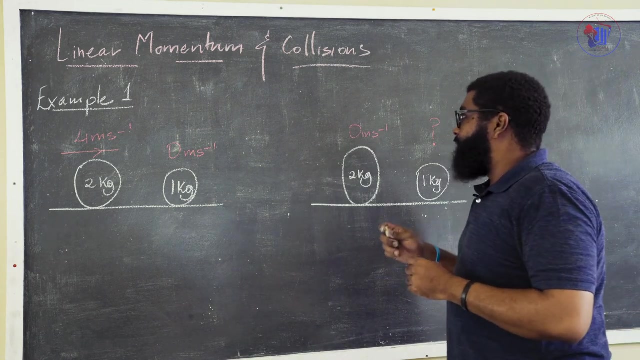 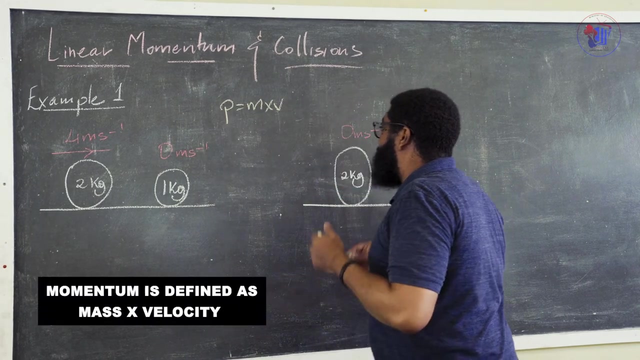 again another zero meter meters, sorry per second, and this is also not moving, but over here we have a question mark, meaning we do not know what happens to this one kilogram mass. well, let's find out. so if we remember from last lesson, we define momentum as mass by velocity. it would imply that 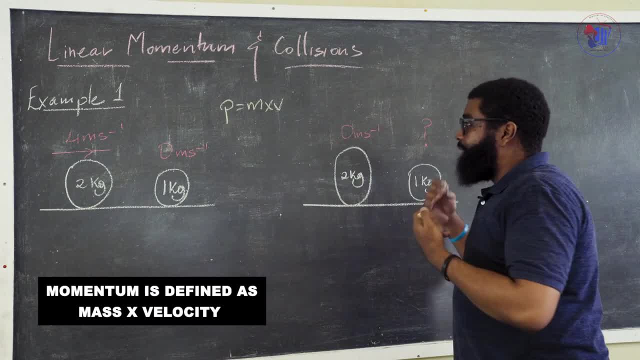 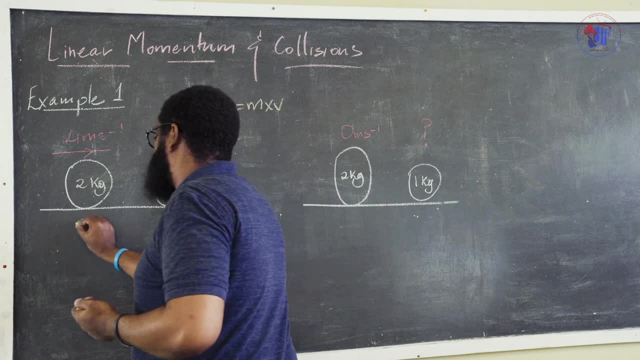 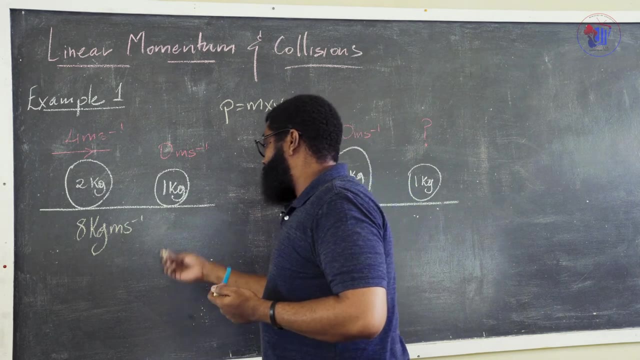 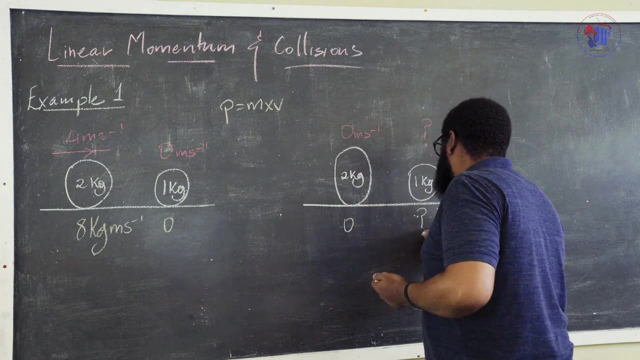 each object, in this entire scenario, has a momentum mass. by velocity, two by four is eight kilogram meters per second. well, one by zero is zero. two by zero is zero and we have no clue what happens here because we do not know the velocity. so this question mark: 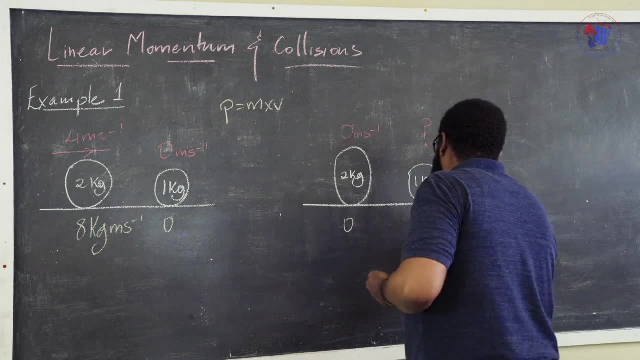 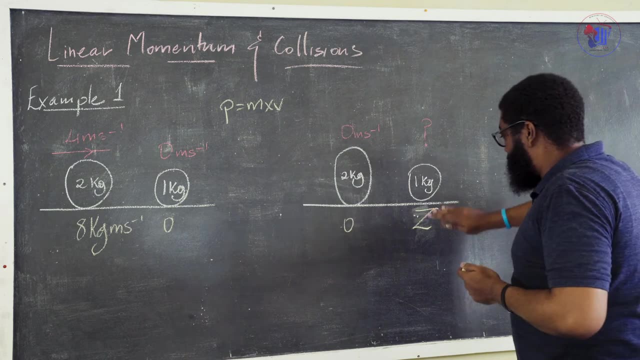 you know what this is not. this is not a good idea. let me not use a question mark. let's call the momentum of the one kilogram mass zed. yes, okay, the question mark is velocity and i don't want to confuse anyone at home. so the question mark. 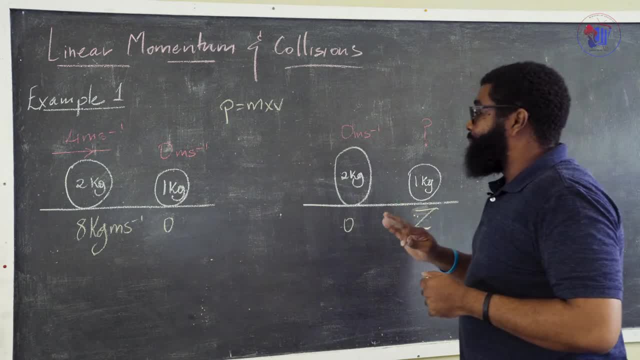 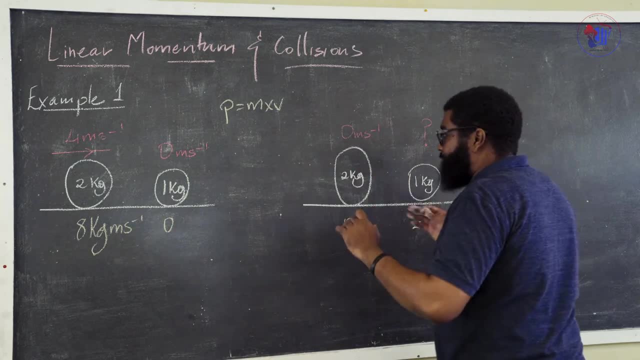 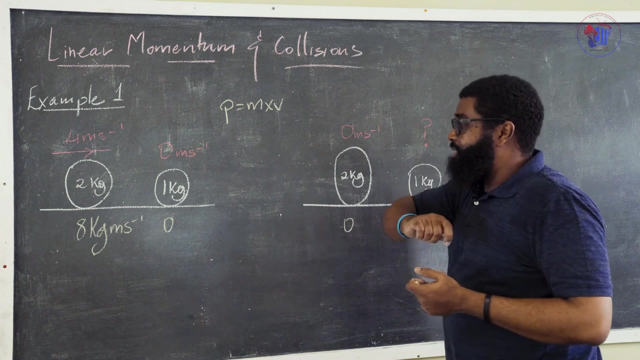 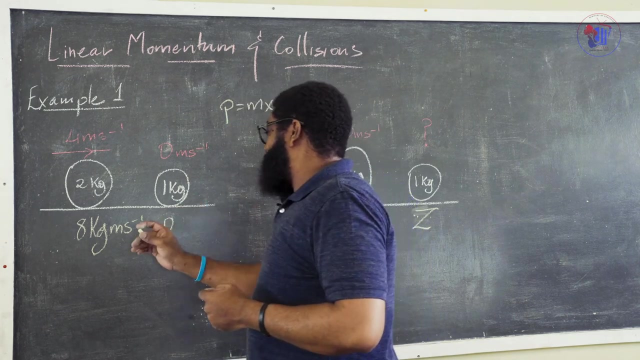 is velocity, the unknown momentum is zed so by the principle of conservation of momentum. if we add up these values, and we add up this value, they should be the same: total momentum before, total momentum after. and the assumption is made is elastic. now some math for you. this here, i will assume that this is positive. okay, now i will by saying this: 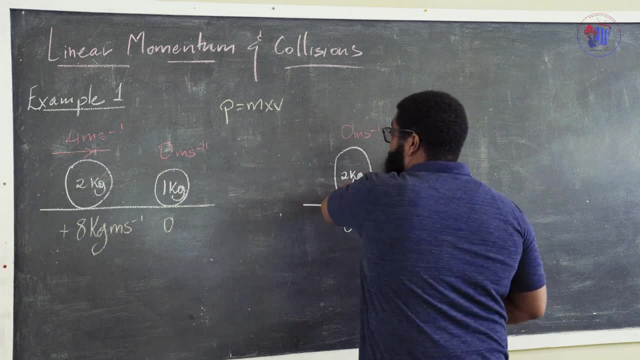 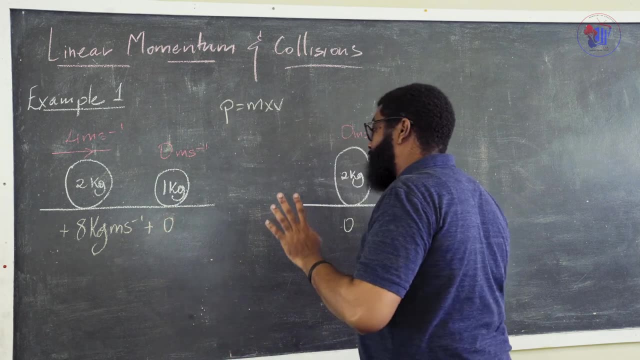 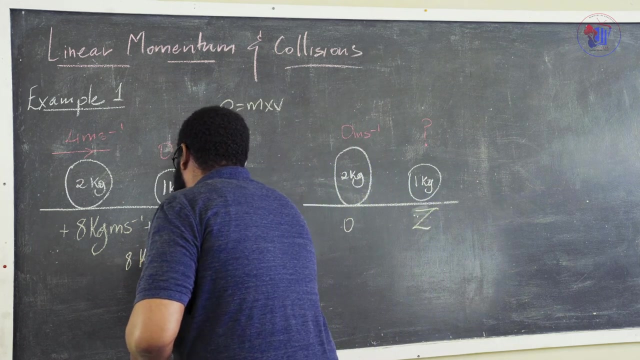 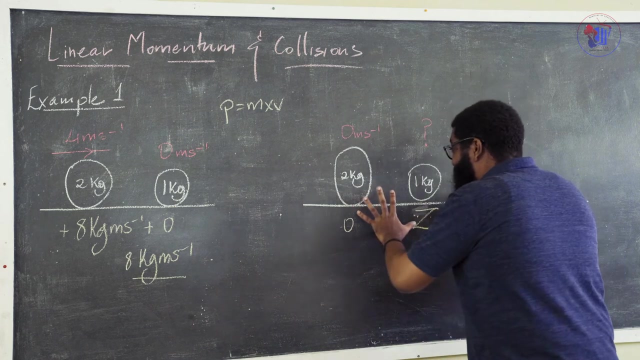 is positive. it means that this direction going to your right is positive. okay, i'm going to add this here and my total on the side- this side, which is the total before they collide- is eight kilogram meters per second. now it means that my total on this side, by the principle of 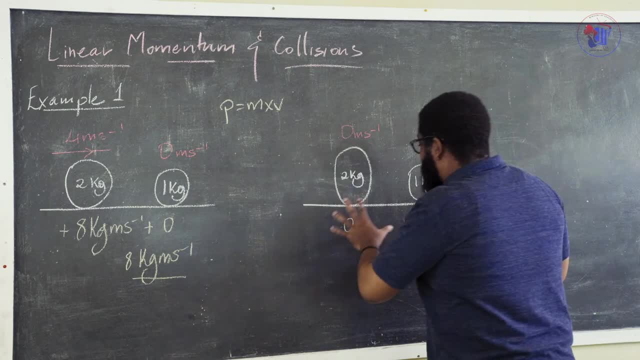 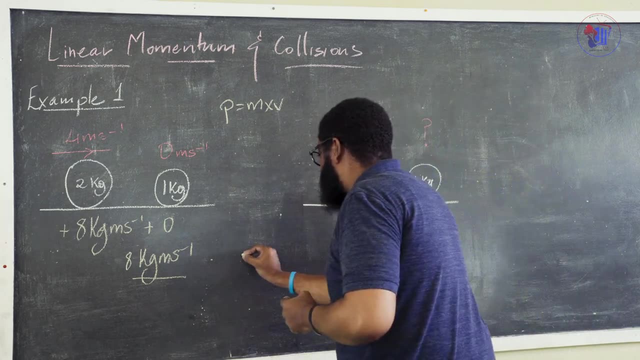 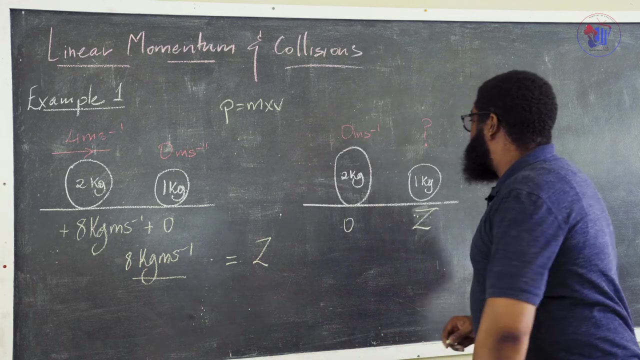 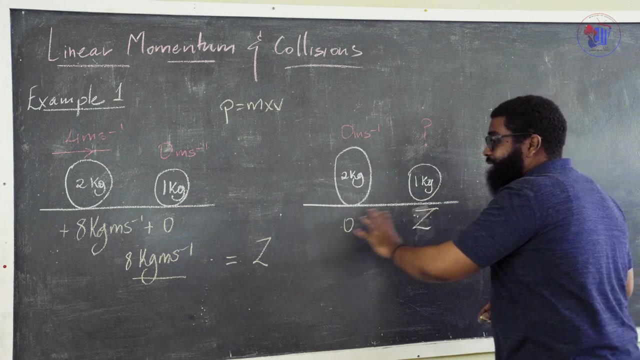 conservation of linear momentum. take a breath before you say it. the total here should be eight as well. so my limited mathematic skills tell me that zero plus zed is the same as just zed, because i would have to give you an example. so what does that mean? because zed is positive. 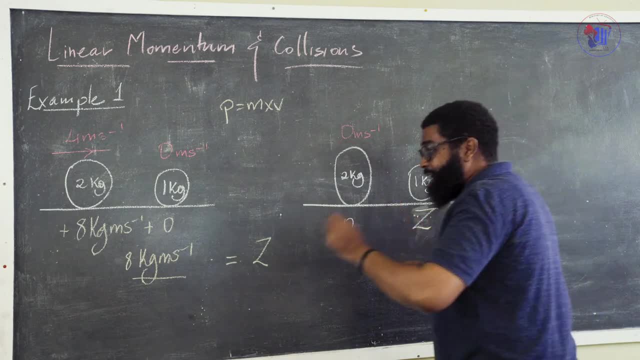 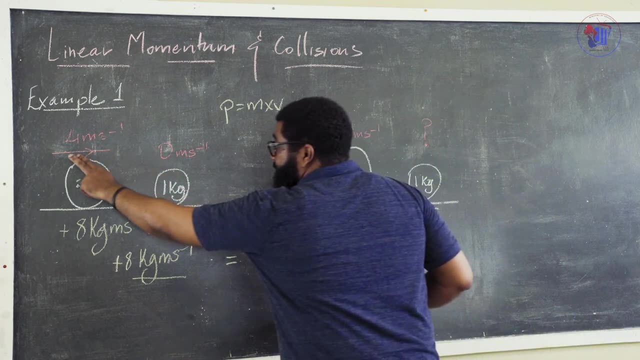 so this: the zed is positive. it tells me that zed is moving in the same direction as zed. and so the zed is positive. so what i have here? i move it in the same direction as zed. it shows me that zed is moving in the same direction as zed in just one second. 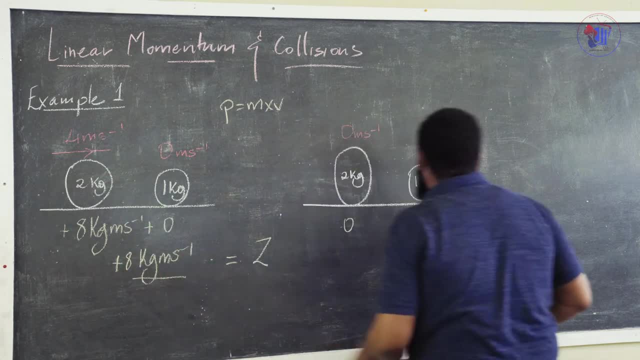 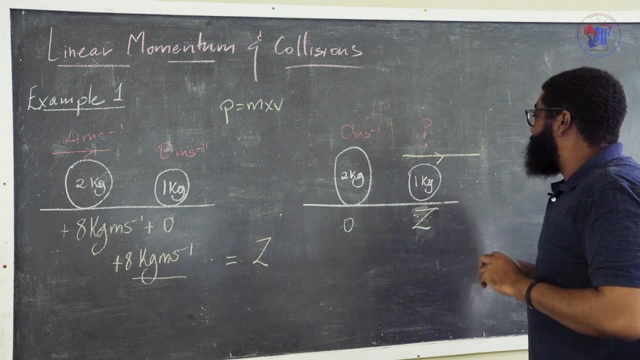 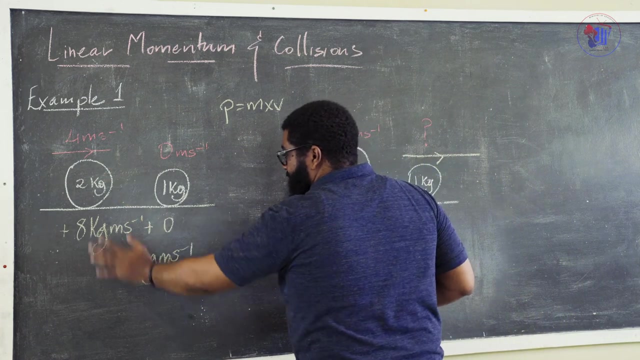 so what i have here is from the momentum of this object, which is represented by the letter z, the momentum of my one kilogram mass direction, which is the positive direction. now, please note, i didn't take it as positive because of the number line, i just took it as positive because it was the only value we had over here. 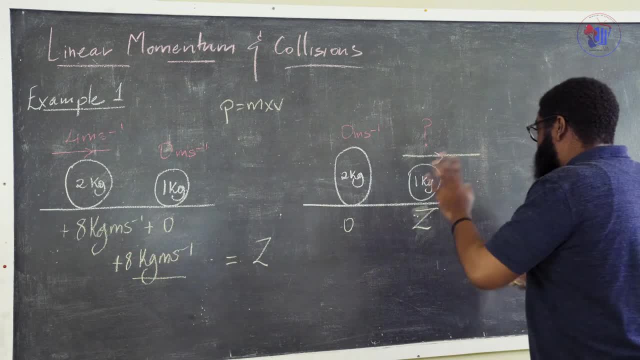 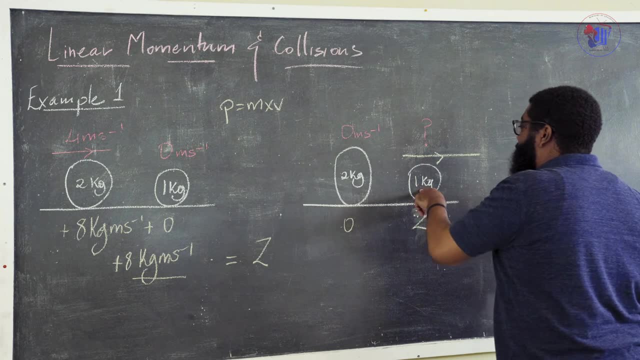 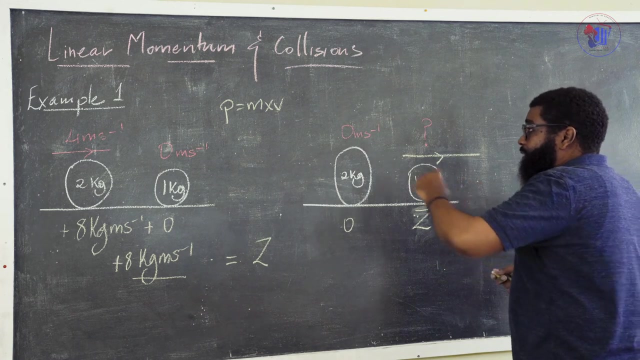 that was a non-zero value. just it has nothing to do with the number line, so just putting that out there. so this z is the momentum of the one kilogram mass. but my unknown here, the question mark was really asking not for momentum but it was asking for velocity. now looking at this equation: 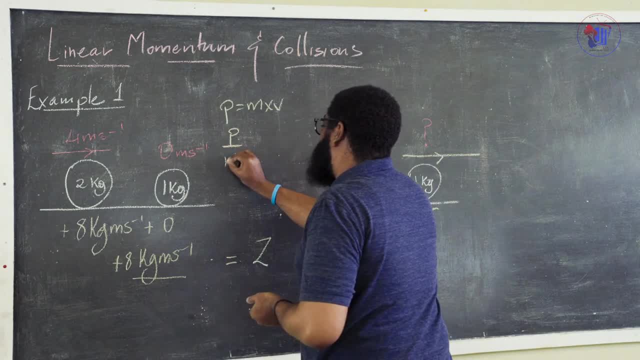 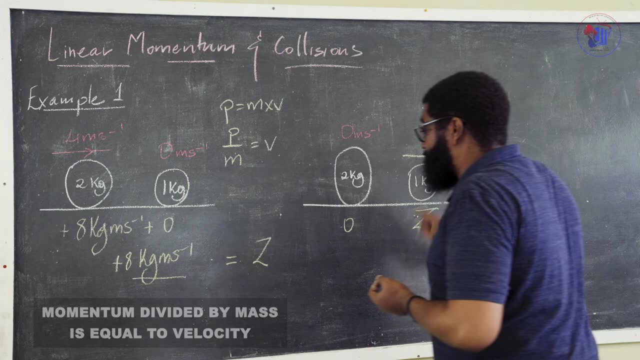 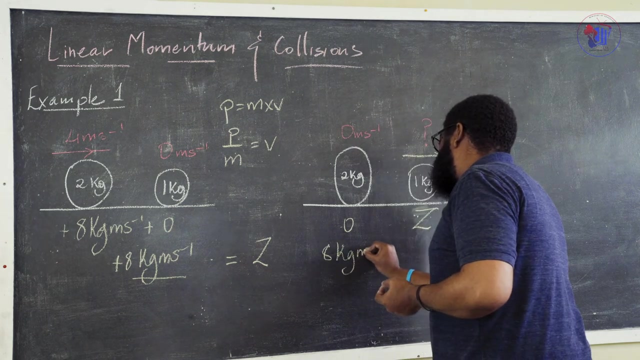 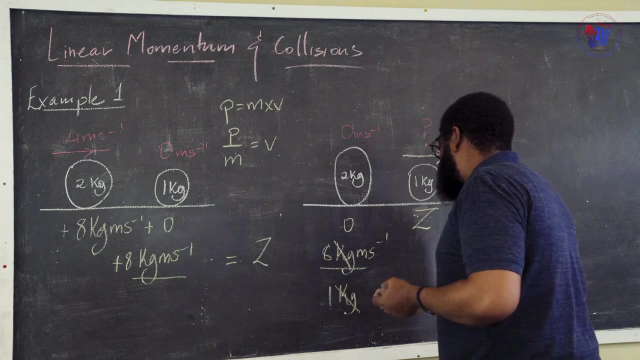 we can easily see that momentum divided by mass gives us velocity. so the velocity of this, the velocity of our one kilogram object, will be equal to momentum. eight kilogram meters, a second divided by one kilogram. yes, the units do cancel out and the answer we get is eight meters per second. so this velocity, 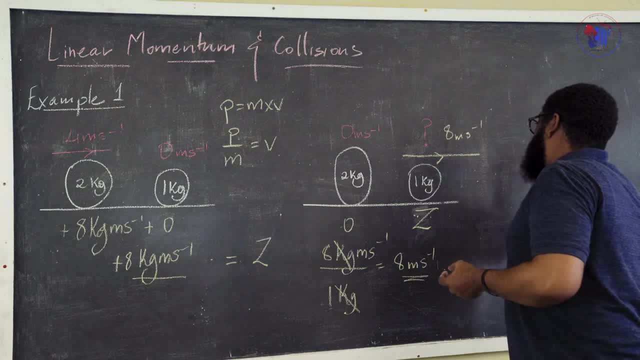 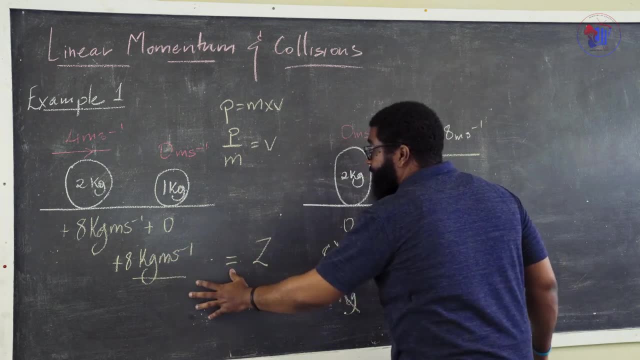 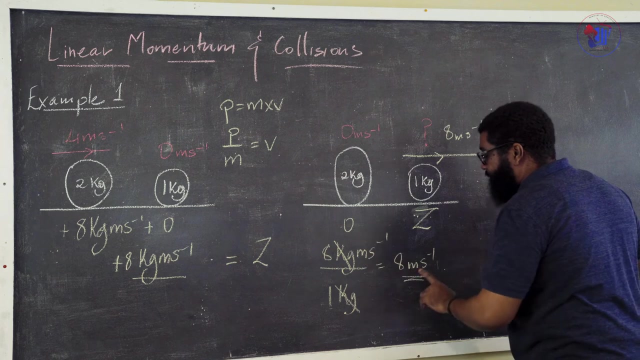 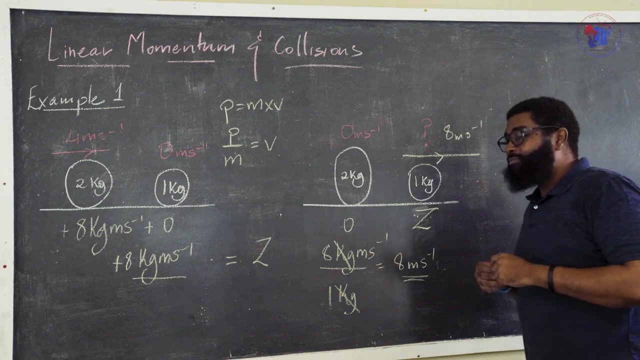 would be eight meters per second in that direction. simple, total momentum before, total momentum after. this applies because the collision is assumed to be elastic and we simply rearrange this formula, use it here to get our value of velocity, which is eight meters per second. and this is our first example. you can always check, oh, please check, and you can even make up your. 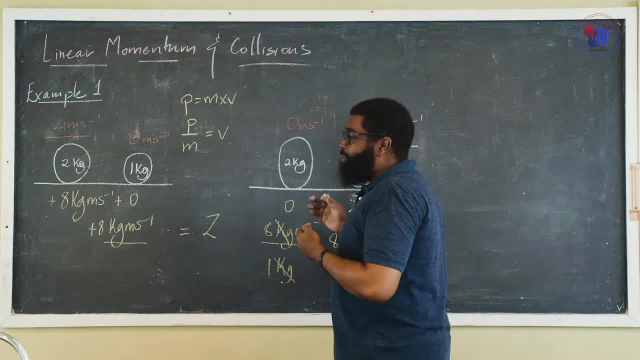 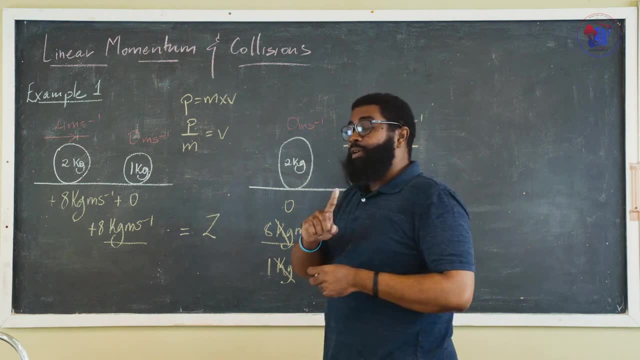 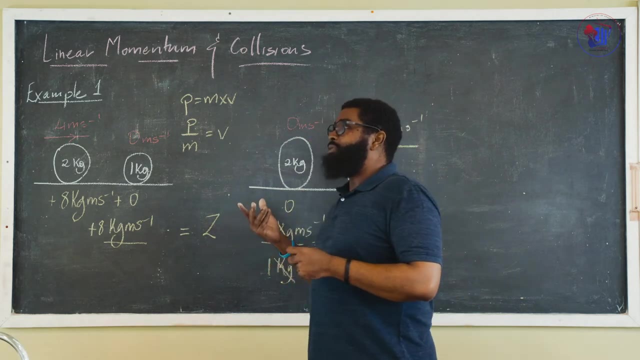 own examples, if you want, and change the numbers around, but you're going to see that it should work out or it should be worked this way: um. now, before i move on there, there are times when um, a formula is given: um, m1, v1 plus m2, v2 is equal to something. i hope i'm getting it right. 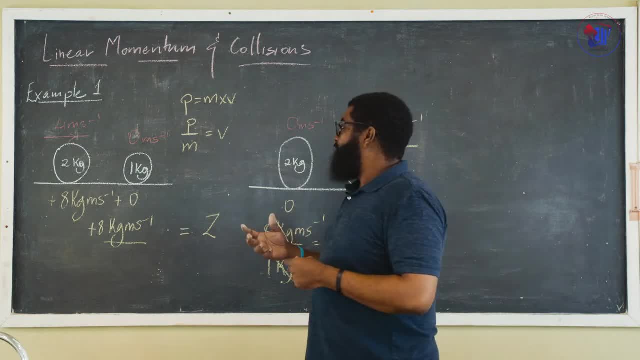 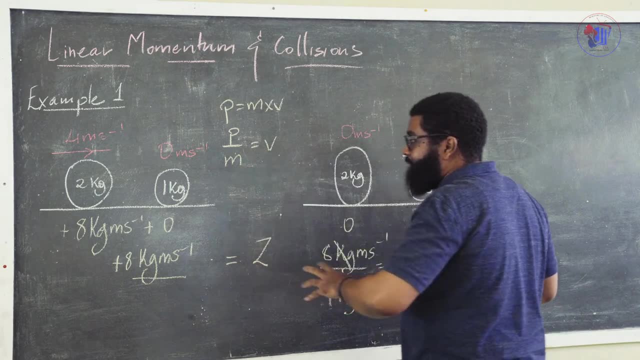 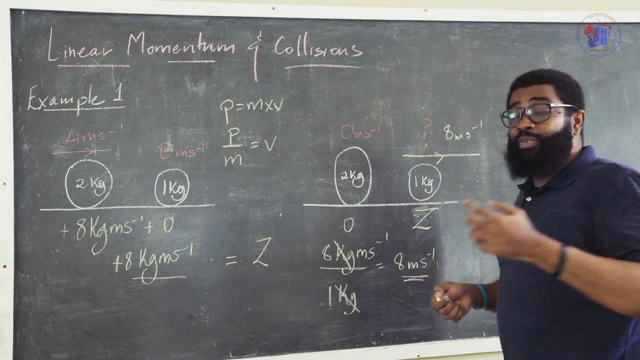 but i usually avoid the formula for the simple reason that, um, it pays to actually be able to analyze the situation on its merit, because sometimes that formula doesn't always help, because there's some scenarios where you can even start off with a single object and then you end up. 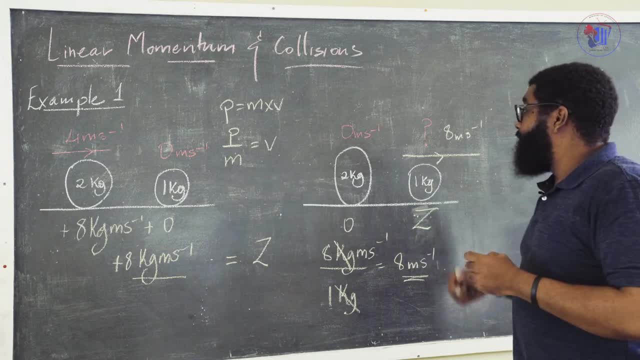 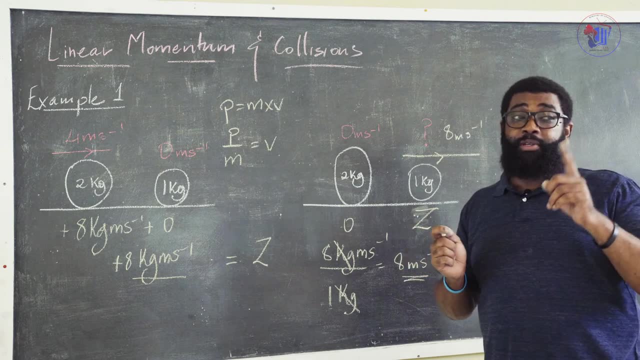 with two separate parts. yeah, that's actually an example and we will look at it. i think that will be our last example, so for now, folks do check over, tell me if i'm right and let's move on to example number two. having changed the color of my chalk. 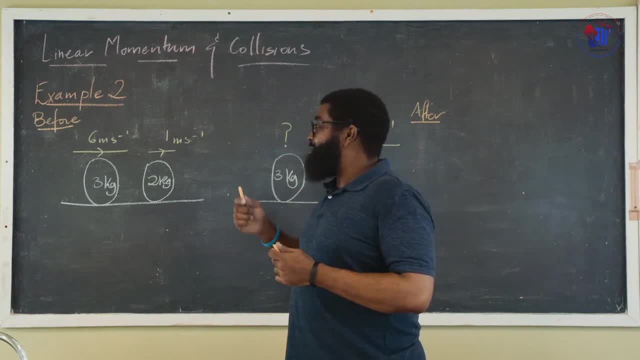 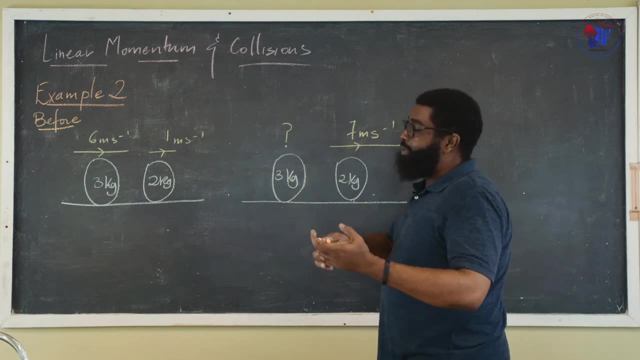 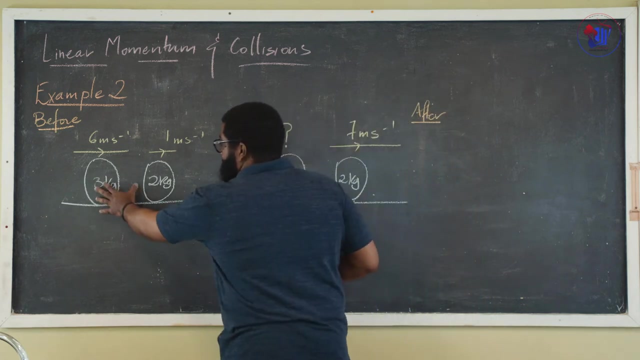 and through the power of editing, i guess. um, this is the second example now. the first example: we had one object at rest and the other one hit it and then that one came to rest and first object that was at rest, you know, moved off. here is different. we have two objects, one moving at six. 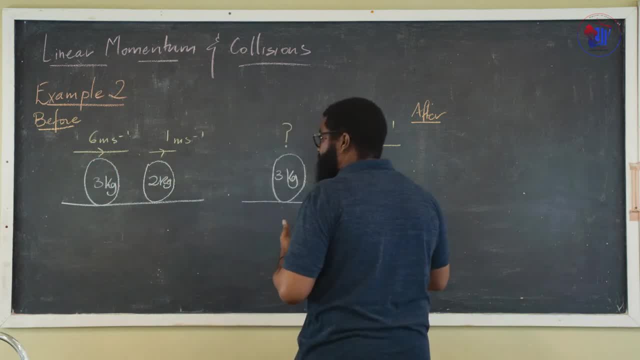 meters per second to the right, the other moving six meters per second, two moving by five meters second to the right as well, and they collide. now, just so you might be wondering: like why did they collide? um, sorry, i said, i said six meters per second for both. um, i think. anyways, this is way. 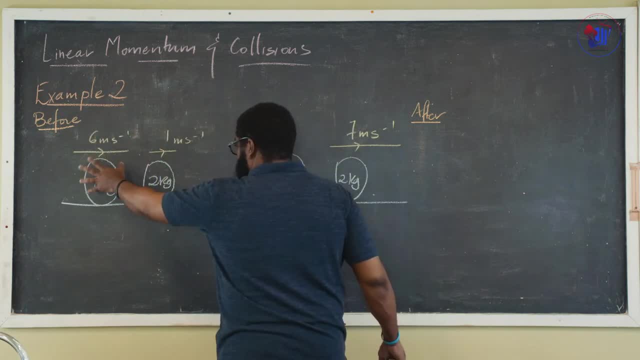 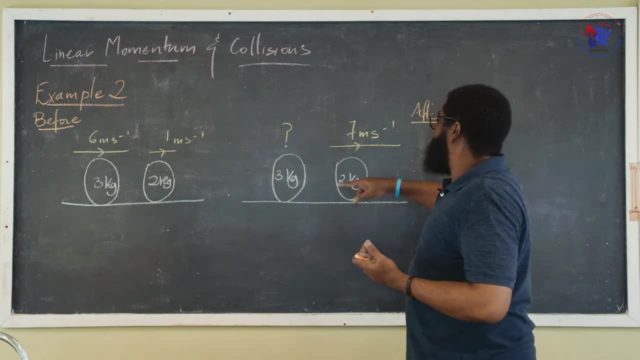 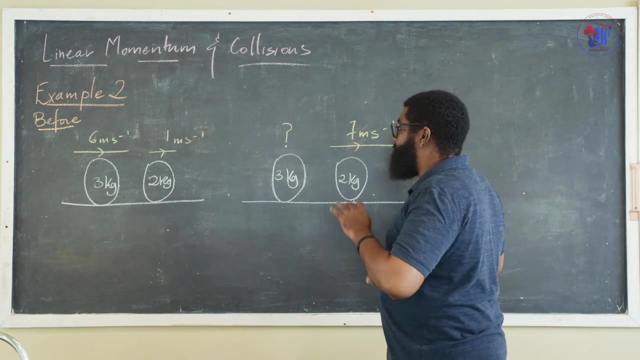 faster than that, all right. so essentially, one runs into the other from behind. that's. that's what happens. now, after they collide, the two kilogram mass has a very large increase in velocity. we want to find out what happens to the three kilogram mass. so again, principle of conservation. 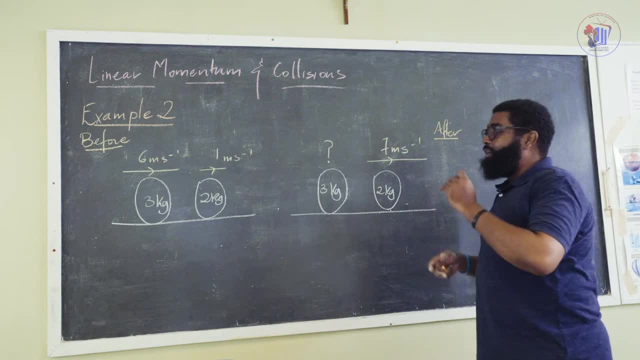 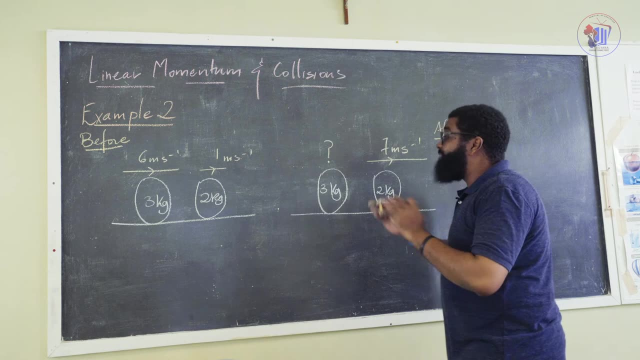 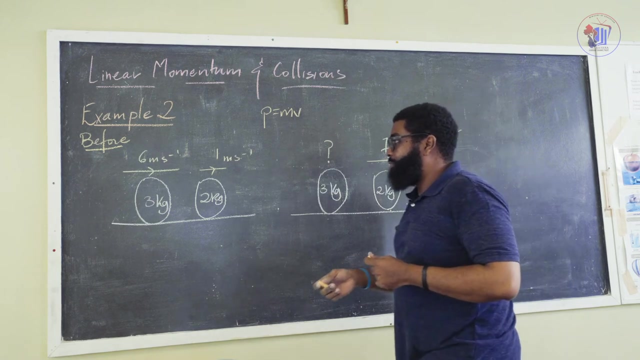 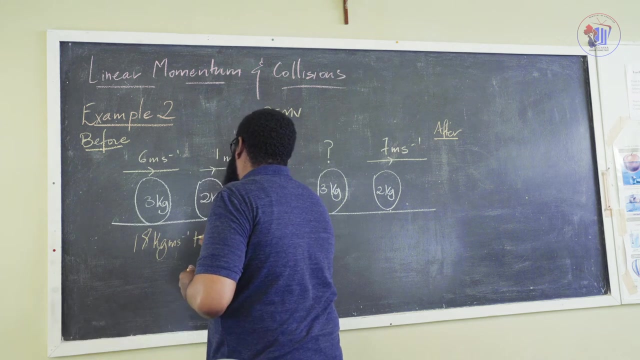 of linear momentum is applied because we assume the collision to be elastic. kinetic energy before is equal to total kinetic energy after um, and we never, ever lose sight of this. momentum is mass by velocity. so six by three is 18 kilogram meters per second, plus two by one. mass by velocity: two, ones or two. 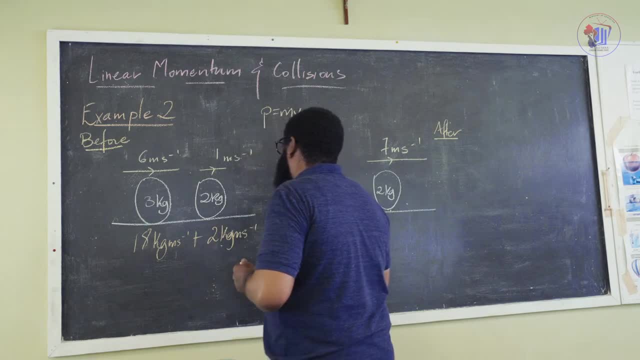 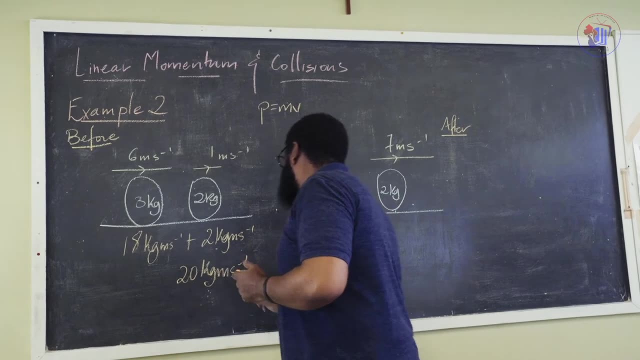 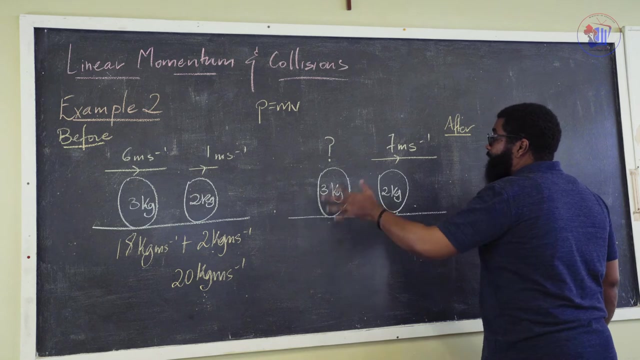 and let me see: magically, 18 and two give us 20 kilogram meters per second. now it means that this 20 kilogram meters per second should be the total momentum of these two objects after they collide. again, we assumed the collision to be elastic. kinetic energy before and after they collide, so we assume the collision to be elastic. 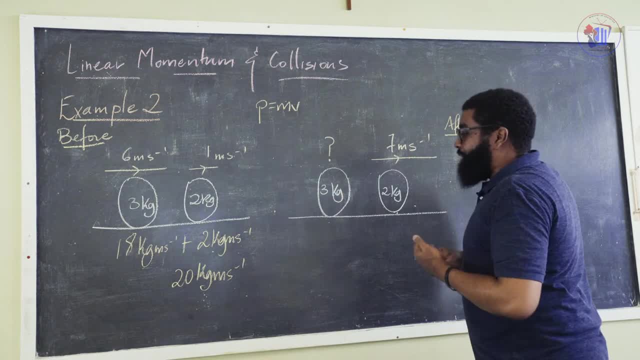 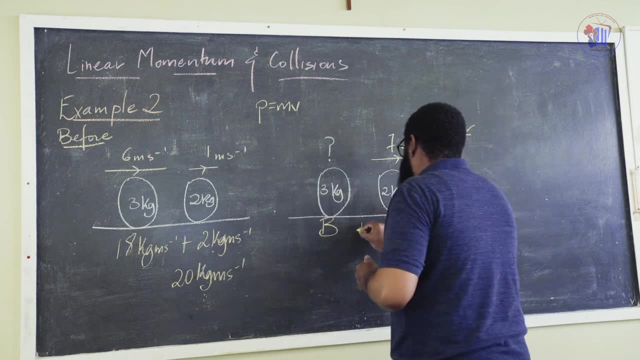 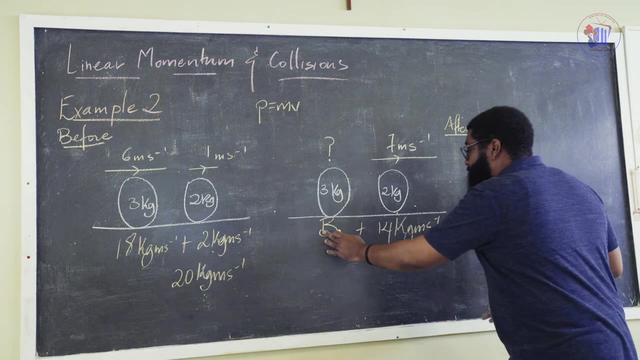 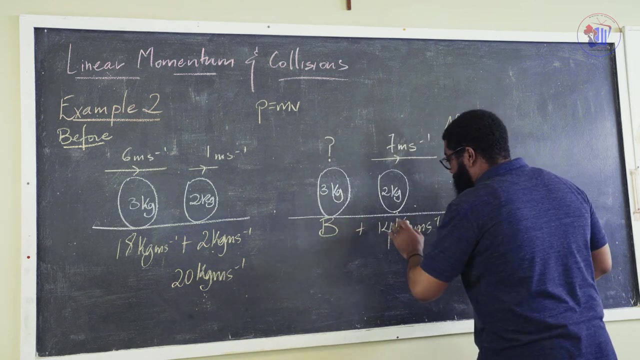 so let's call the momentum of the three kilogram mass b. okay, b two sevens are- last i checked- 14. good, so it implies that b plus 14 is 20. in other words, 20 is equal to b plus 14, now in primary. 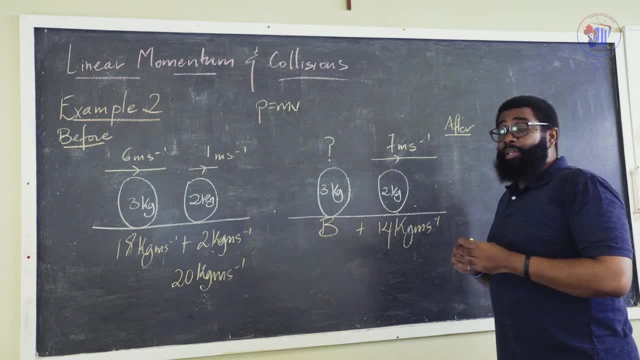 school, when we were given questions like this: if we got them wrong, we would have to do the same thing again. so we would have to do the same thing again. we would have to do the same thing again. so we would have to do the same thing again. so we would have to do the same thing again. 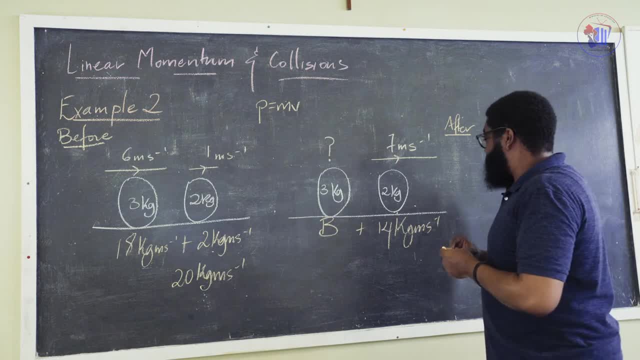 we would have to do the same thing again. so we would have to do the same thing again. so we would have to do the same thing again to get a couple lashes. i hope i don't deserve lashes for getting this one wrong. to get a couple lashes. i hope i don't deserve lashes for getting this one wrong. 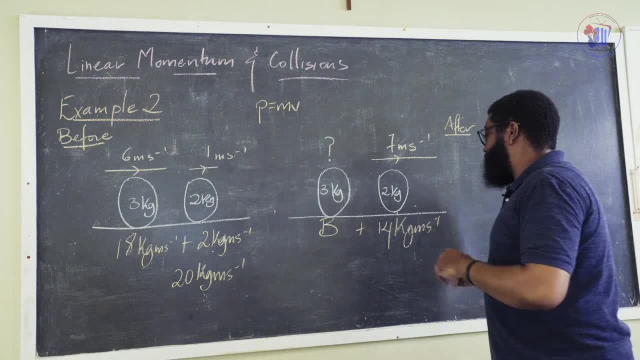 to get a couple lashes. i hope i don't deserve lashes for getting this one wrong. um this b is six kilogram meters per second. um this b is six kilogram meters per second. um this b is six kilogram meters per second because six plus 14 would give us 20.. if we 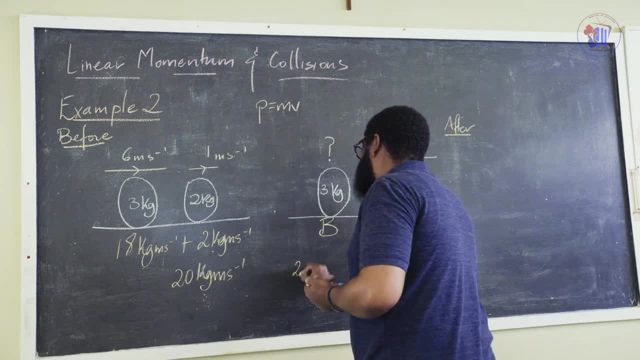 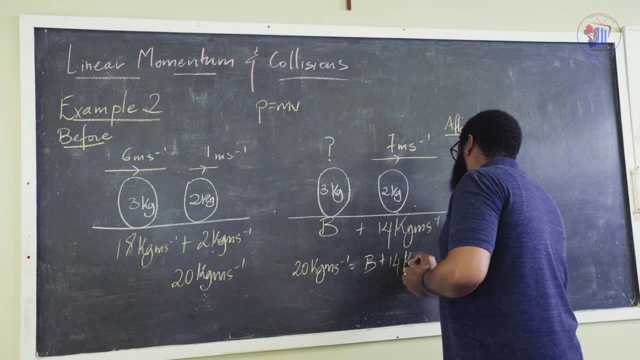 because six plus 14 would give us 20.. if we- because six plus 14 would give us 20.. if we want to do it the correct way, we could want to do it the correct way, we could want to do it the correct way, we could write it out. 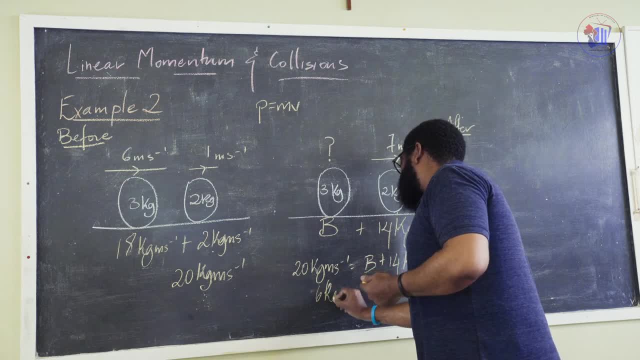 when we do the transposition, we end up when we do the transposition, we end up when we do the transposition, we end up with six kilogram meters per second, with six kilogram meters per second, with six kilogram meters per second is b and that is the momentum. 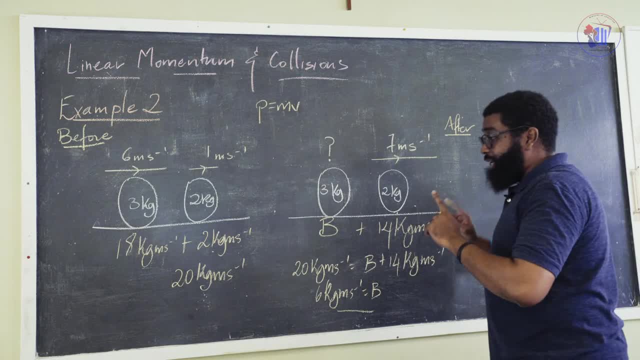 is b, and that is the momentum is b, and that is the momentum of the three kilogram mass, again of the three kilogram mass, again of the three kilogram mass, again, again. since these two objects, again, since these two objects, again, since these two objects are traveling well in the same direction. 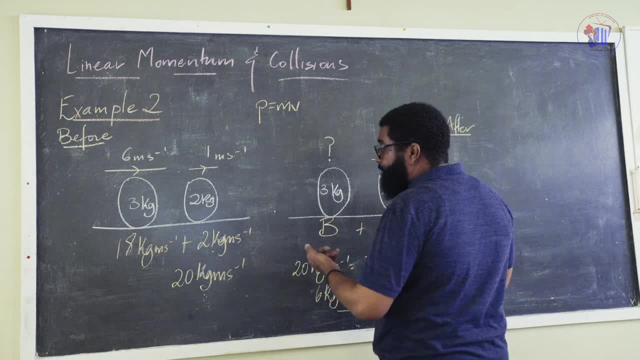 are traveling well in the same direction, are traveling well in the same direction. we add the momentum of the two. we add the momentum of the two. we add the momentum of the two. we don't need to subtract anything. we don't need to subtract anything. we don't need to subtract anything because they're not going in opposite. 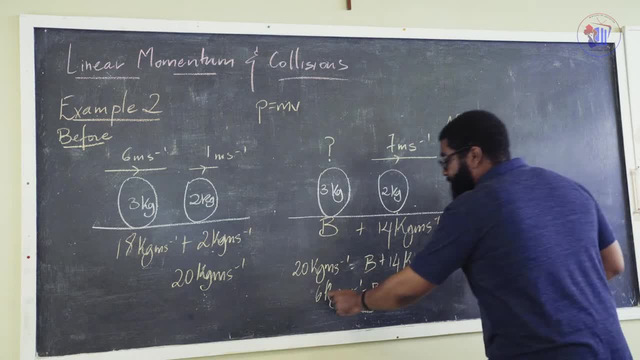 because they're not going in opposite, because they're not going in opposite directions, directions, directions. now, since this value is positive, now since this value is positive, now since this value is positive, what it implies is that this three, what it implies is that this three, what it implies is that this three kilogram mass, 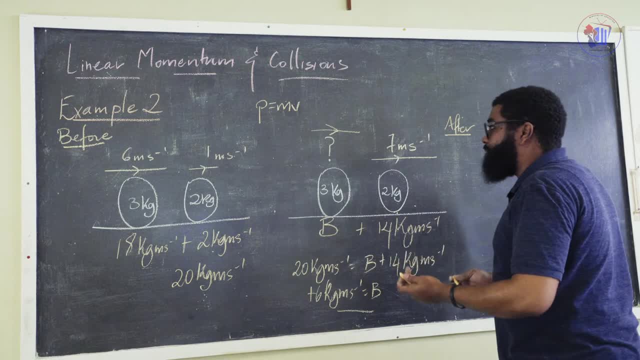 kilogram mass. kilogram mass is moving in the direction, like is moving in the direction, like is moving in the direction, like everything else, everything else, everything else, to the right, but to the right, but to the right. but my guess is it's not moving as fast as. 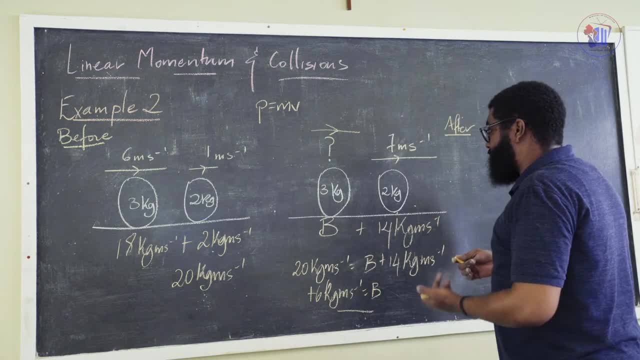 my guess is it's not moving as fast as my guess is it's not moving as fast as it was. it was, it was here. so if i ask what is the velocity here? so if i ask what is the velocity here? so if i ask what is the velocity, which is exactly what this question mark? 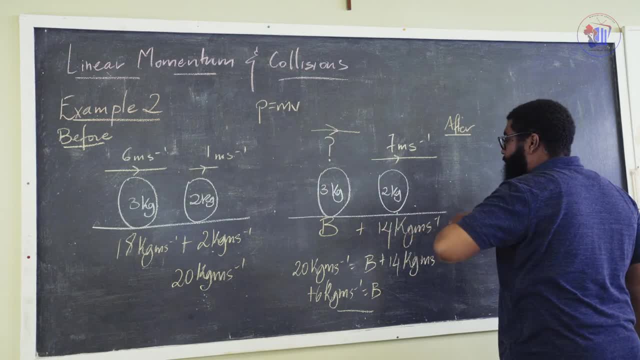 which is exactly what this question mark, which is exactly what this question mark implies: mean, implies, mean, implies, mean. how fast is this thing moving? we, just how fast is this thing moving. we, just how fast is this thing moving? we just rearrange the formula again: momentum. rearrange the formula again: momentum. 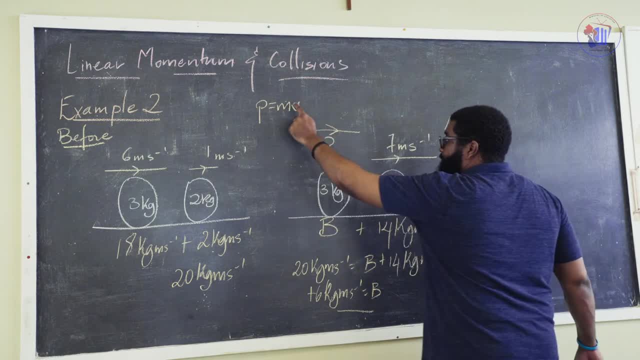 rearrange the formula again. momentum p is mass m by velocity v. therefore, p is mass m by velocity v. therefore p is mass m by velocity v. therefore, velocity v would be momentum p divided. velocity v would be momentum p divided. velocity v would be momentum p divided by mass m. momentum is six. 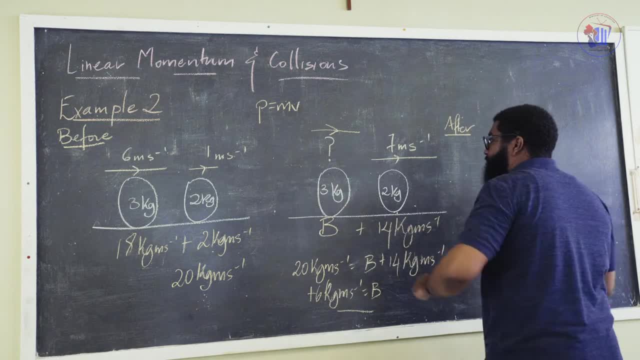 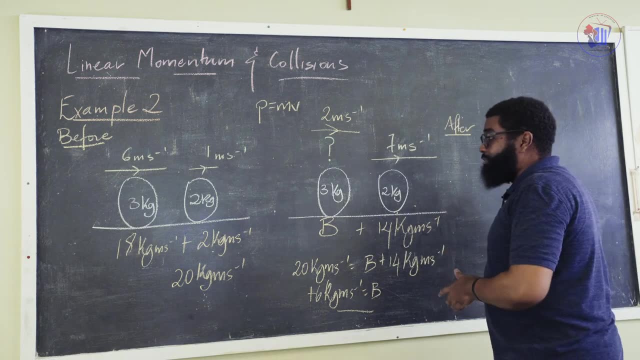 by mass m momentum is six. by mass m, momentum is six. mass is three. six, mass is three. six, mass is three. six divided by three. divided by three, divided by three, would give us, would give us, would give us two meters per second, as we can clearly see. 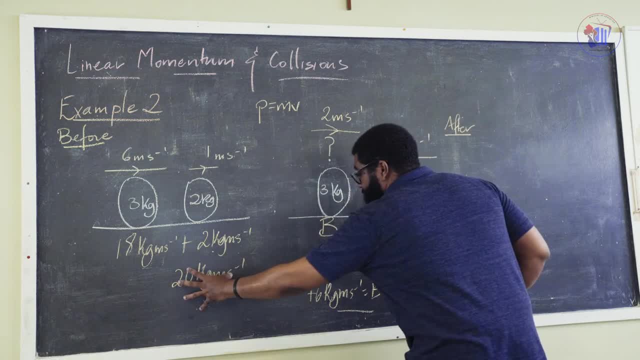 as we can clearly see, as we can clearly see if we do the math, if we do the math, if we do the math, the total momentum here, the total momentum here, the total momentum here is equal to the total, is equal to the total, is equal to the total momentum here, because we assume the 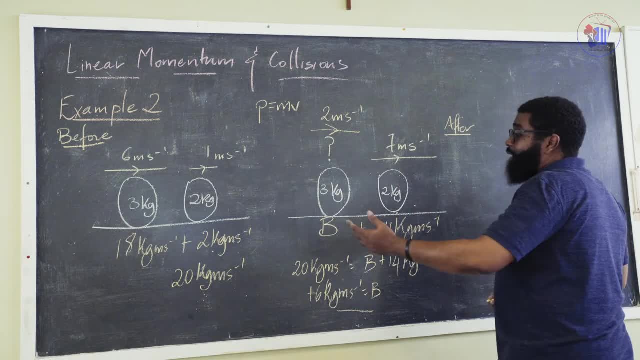 momentum here. because we assume the momentum here, because we assume the collision to be elastic, collision to be elastic, collision to be elastic, and our directions are all to the right and our directions are all to the right and our directions are all to the right because all our values are positive and 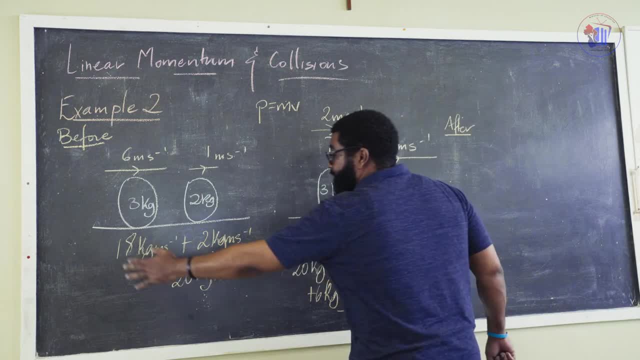 because all our values are positive and because all our values are positive. and again, again, again. it has nothing to do with the number. it has nothing to do with the number. it has nothing to do with the number. line i could have said, line i could have said: 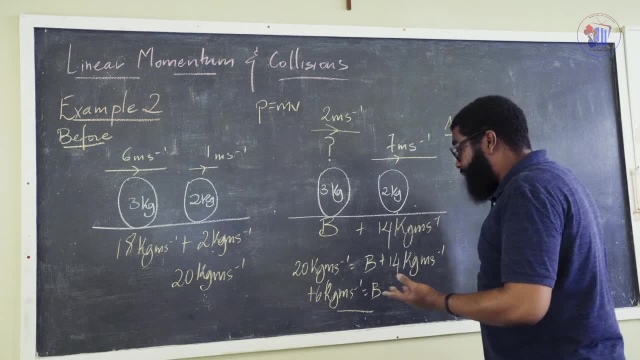 line. i could have said minus 18 minus 2 minus 20.. i could have minus 18 minus 2 minus 20.. i could have minus 18 minus 2 minus 20.. i could have done that, done that, done that, and over here i would have had minus 6. 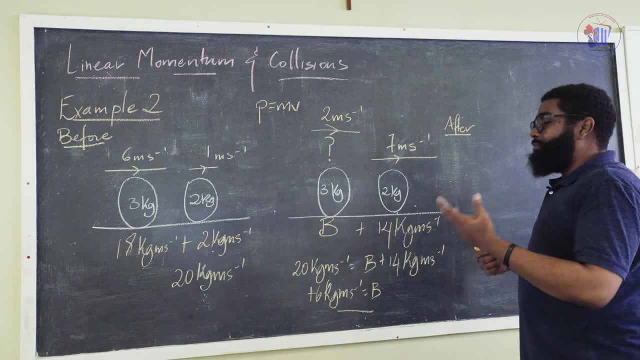 and over here i would have had minus 6, and over here i would have had minus 6 and minus 14.. you can take any direction, and minus 14.. you can take any direction, and minus 14.. you can take any direction: going to the left or going to the right. 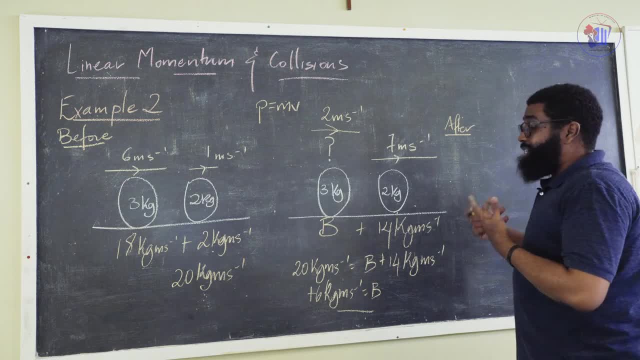 going to the left or going to the right, going to the left or going to the right, as positive, okay. it doesn't matter. as positive, okay, it doesn't matter. as positive, okay, it doesn't matter. i just find it easier to work with. i just find it easier to work with. 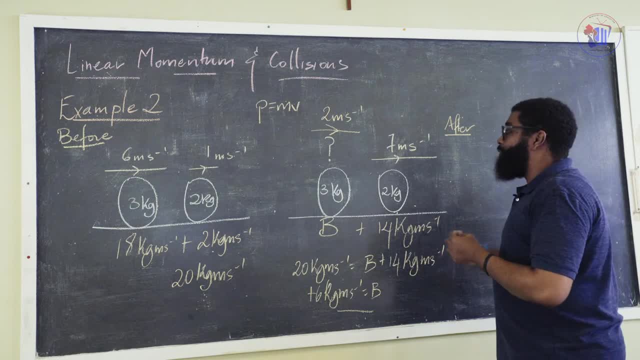 i just find it easier to work with positive numbers, positive numbers, positive numbers. so the principle of conservation of, so, the principle of conservation of, so the principle of conservation of linear momentum, linear momentum. linear momentum helped us to find the momentum b, which helped us to find the momentum b which 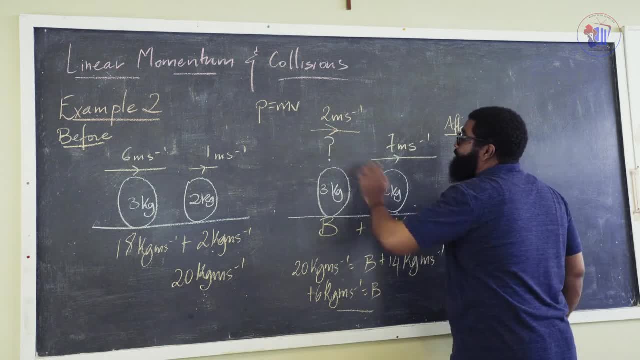 helped us to find the momentum b, which is six kilogram meters per second. is six kilogram meters per second. is six kilogram meters per second, and our velocity, which is two meters per, and our velocity, which is two meters per, and our velocity, which is two meters per second. 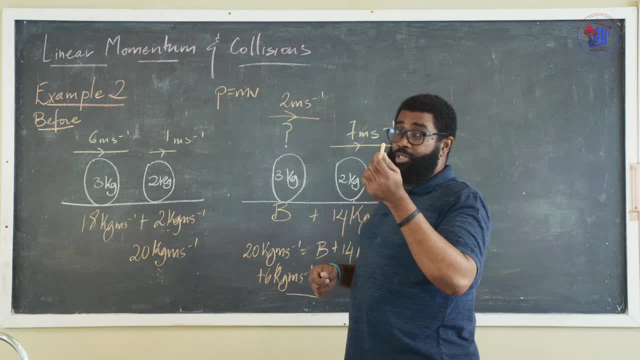 second, second. this is our second scenario. so this is our second scenario. so this is our second scenario. so do check over ensure i'm right. i will do check over ensure i'm right. i will do check over ensure i'm right. i will change the color of my chalk write. 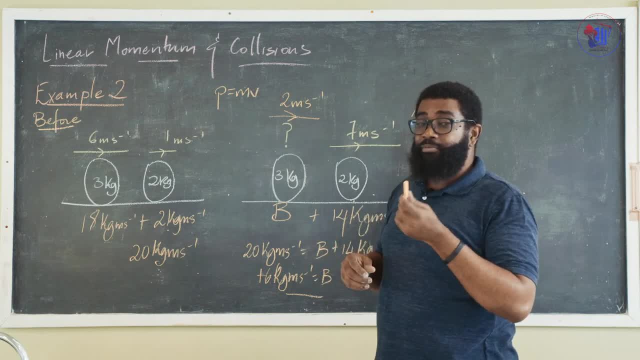 change the color of my chalk. write: change the color of my chalk. write. another example on the board. another example on the board. another example on the board. we have two more to do. see you just now. we have two more to do. see you just now. we have two more to do. see you just now, having changed the color of my chalk. 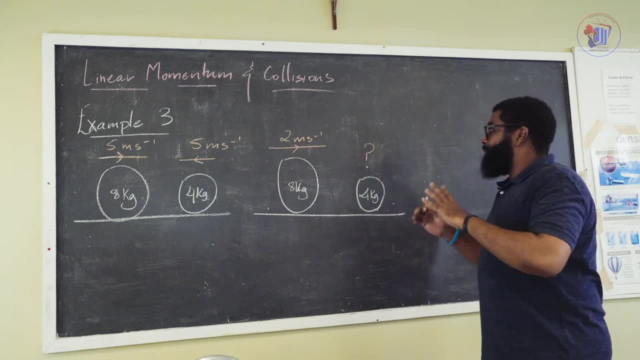 having changed the color of my chalk, having changed the color of my chalk, again, we come back with the third again. we come back with the third again, we come back with the third example now, um, the first example, quickly example. now um, the first example, quickly example. now, um, the first example, quickly recapping, was one object hitting a. 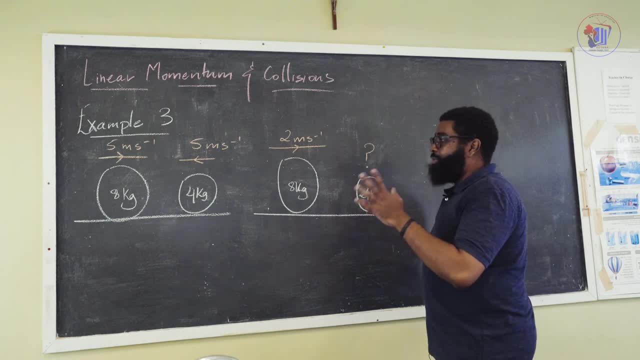 recapping was one object hitting a recapping was one object hitting a stationary object. stationary object, stationary object. this example is just two objects. this example is just two objects. this example is just two objects traveling in opposite directions. now for traveling in opposite directions. now for traveling in opposite directions. now for fun. i used easy numbers. i used the same. 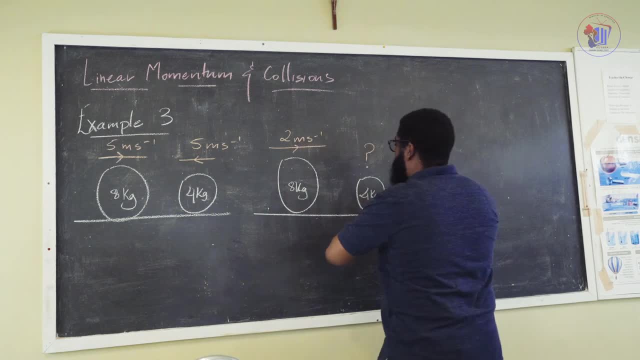 fun. i used easy numbers. i used the same fun. i used easy numbers. i used the same velocity: velocity, velocity. and then we have what happens after the, and then we have what happens after the, and then we have what happens after the collision and our collision and our. 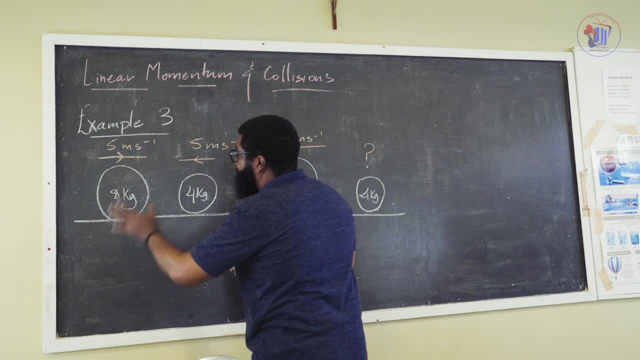 collision and our little unknown. so starting with what little unknown? so starting with what little unknown? so starting with what happens before they collide- happens before they collide- again momentum. i'ma write it for the again momentum. i'ma write it for the again momentum. i'ma write it for the third time. 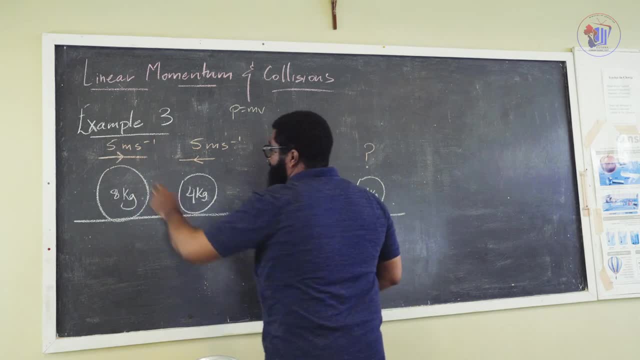 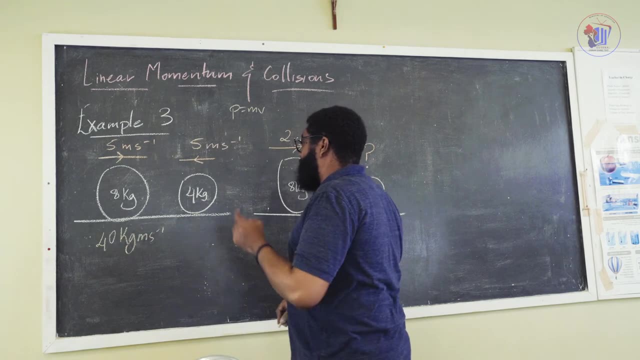 third time. third time: mass by velocity mass. mass by velocity mass. mass by velocity mass times velocity eight fives. last i times velocity eight fives. last i times velocity eight fives. last i checked is 40. checked is 40. checked is 40 kilogram meters per second. okay, 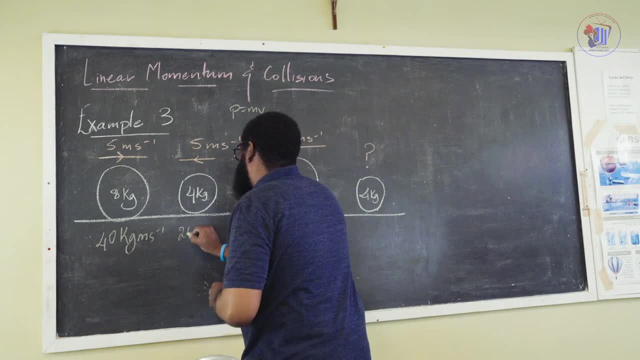 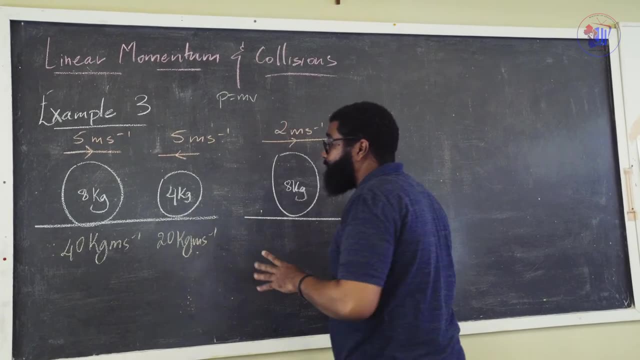 kilogram meters per second. okay, kilogram meters per second. okay, now now now. mass by velocity: four fives are 20. mass by velocity: four fives are 20. mass by velocity: four fives are 20 kilogram meters per second. you would notice that i have put no sign. 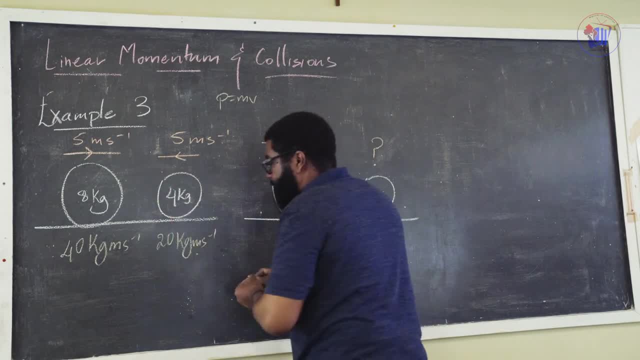 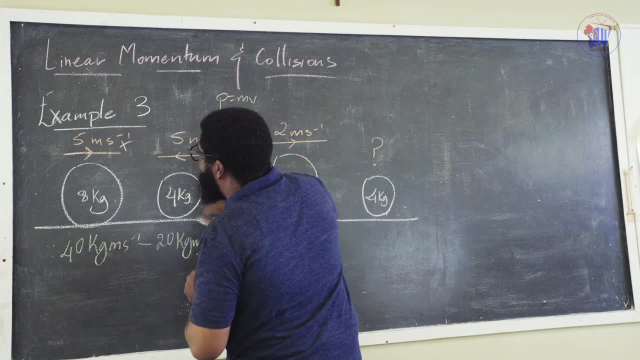 the velocities are in opposite. the velocities are in opposite, the velocities are in opposite directions: directions, directions. therefore, we subtract, therefore, we subtract, therefore, we subtract me. what this means is that i've took me. what this means is that i've took me. what this means is that i've took, i've taken um. 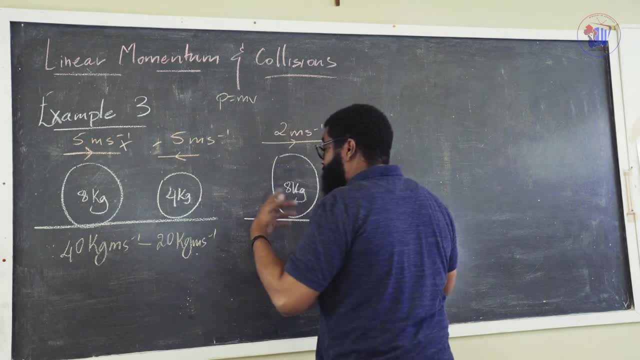 i've taken um. i've taken um. that side is positive and this side will. that side is positive and this side will. that side is positive and this side will obviously be negative, since it's the obviously be negative, since it's the obviously be negative, since it's the opposite direction to that. 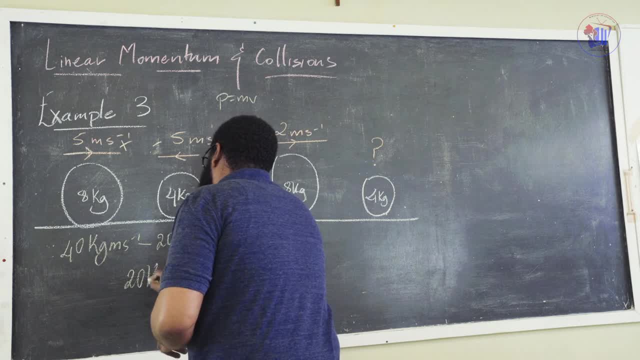 opposite direction to that opposite direction to that. this means 40 minus 20 gives us a grand. this means 40 minus 20 gives us a grand. this means 40 minus 20 gives us a grand. total, total total of 20 kilogram meters per second. 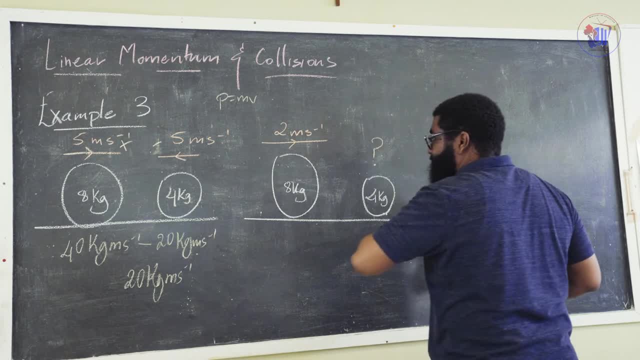 of 20 kilogram meters per second, of 20 kilogram meters per second after they collide, after they collide, after they collide, the eight kilogram mass, the eight kilogram mass, the eight kilogram mass, still moves in the right direct in the, still moves in the right direct in the. 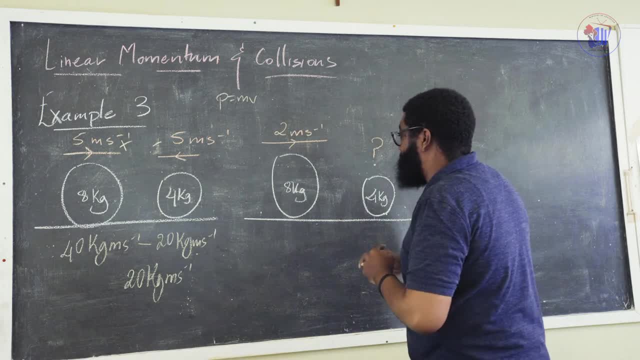 still moves in the right direct, in the right direction, right direction, right direction, with a velocity of two meters per second, with a velocity of two meters per second, with a velocity of two meters per second. so so, so let us see what happens. a, 2 is b. 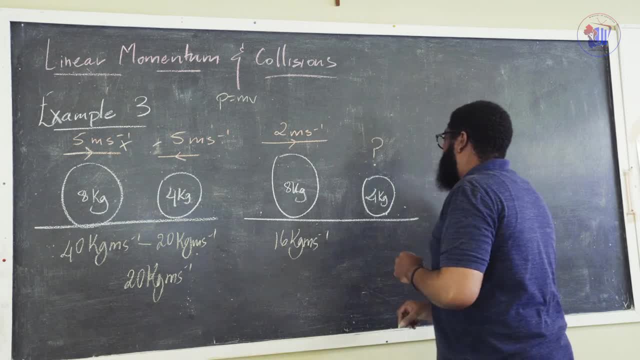 let us see what happens: a, 2 is b. let us see what happens a, 2 is b: 16 kilogram meters per second. 16 kilogram meters per second, 16 kilogram meters per second. and let's call the momentum of the four. and let's call the momentum of the four. 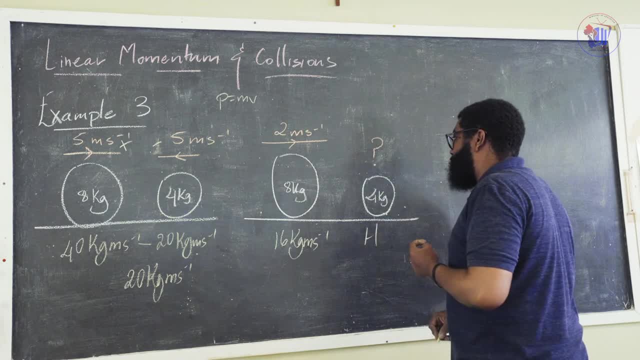 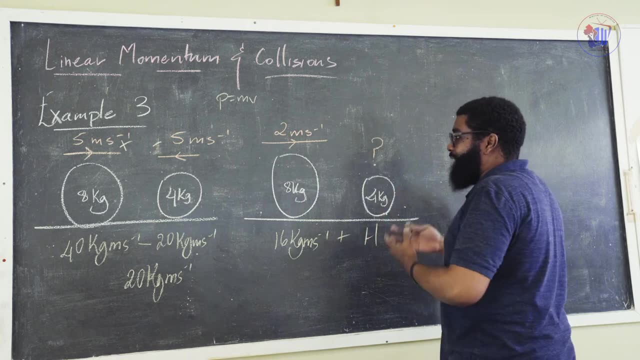 and let's call the momentum of the four: kilogram mass, kilogram mass, kilogram mass: h. so h, so h. so, since it's unknown, you, just since it's unknown, you, just since it's unknown, you just add it, add it, add it again, assuming this collision is elastic. 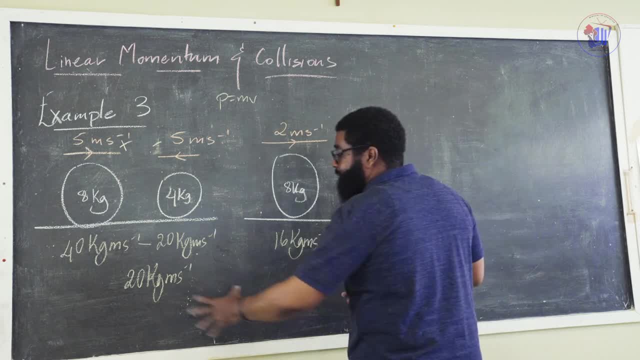 again, assuming this collision is elastic. again, assuming this collision is elastic by the principle of conservation of, by the principle of conservation of, by the principle of conservation of linear momentum, linear momentum, linear momentum. this 20 is equal to this 16 plus h. this 20 is equal to this 16 plus h. 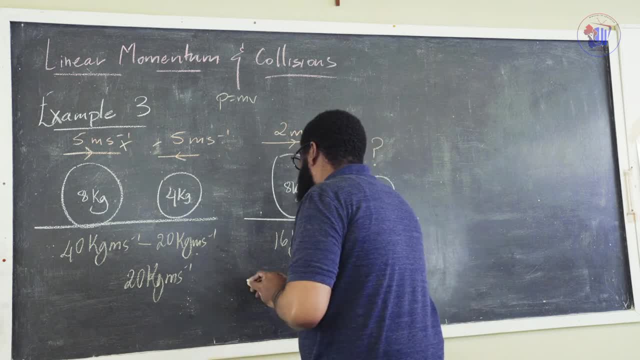 this 20 is equal to this 16 plus h. so so, so, doing a little math, we quickly figure out. doing a little math, we quickly figure out. doing a little math, we quickly figure out that, if 20, that if 20, that if 20 kilogram meters per second. 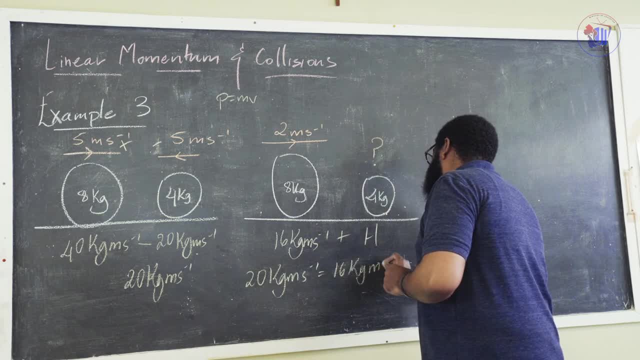 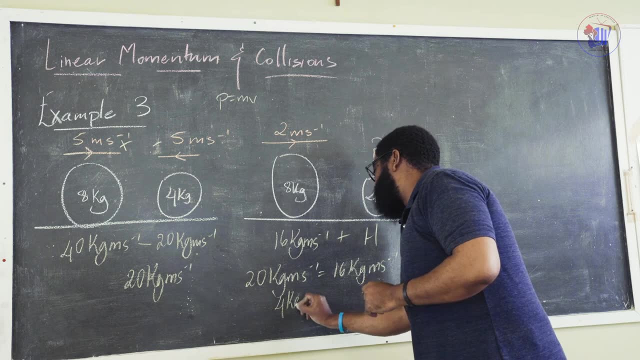 is equal to 16 kilogram meters. per is equal to 16 kilogram meters. per is equal to 16 kilogram meters per second, plus h. it would imply plus h. it would imply plus h. it would imply that h is four, that h is four. 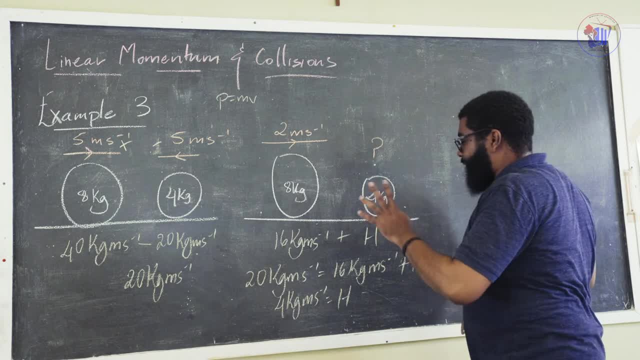 that h is four kilogram meters per second kilogram meters per second. kilogram meters per second. again, we carry this across, again. we carry this across, again, we carry this across: 20 minus 16 gives us four, so the momentum. 20 minus 16 gives us four, so the momentum. 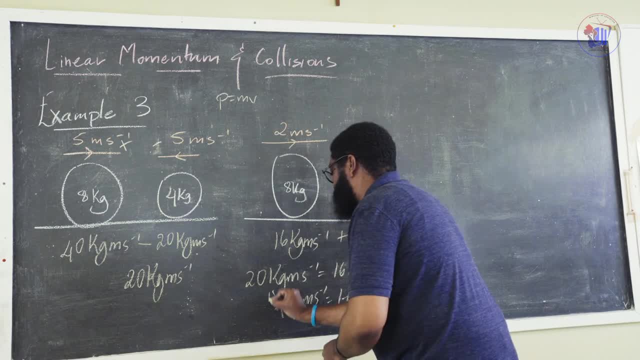 20 minus 16 gives us four. so the momentum of h is four, but please note of h is four. but please note of h is four. but please note it's positive. four plus four, that would it's positive. four plus four, that would it's positive. four plus four, that would mean: 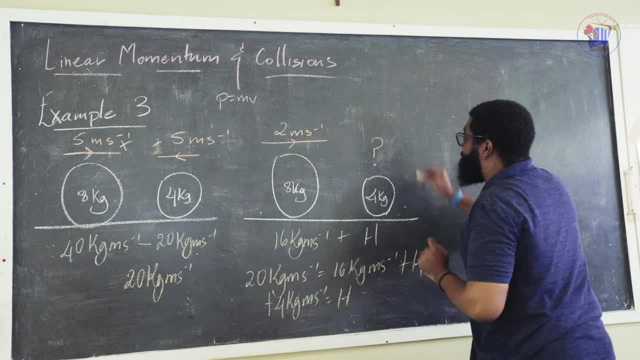 mean mean that this mass is now moving in the, that this mass is now moving in the, that this mass is now moving in the positive direction, positive direction, positive direction. so it's moving to the right and again. so it's moving to the right and again. so it's moving to the right and again. please don't think that- always moving to. 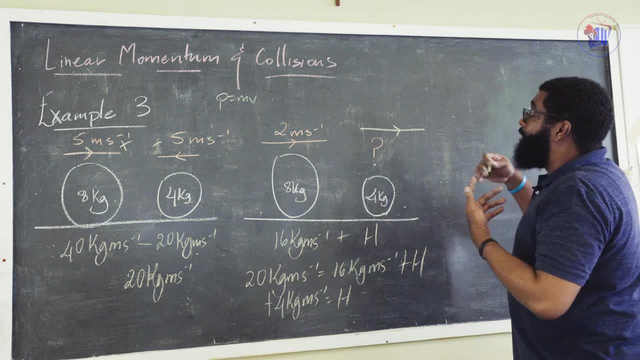 please don't think that always moving to, please don't think that always moving to the right is positive, the right is positive, the right is positive. not the case i just choose, i just choose. not the case i just choose, i just choose. not the case, i just choose, i just choose numbers that give us these values. 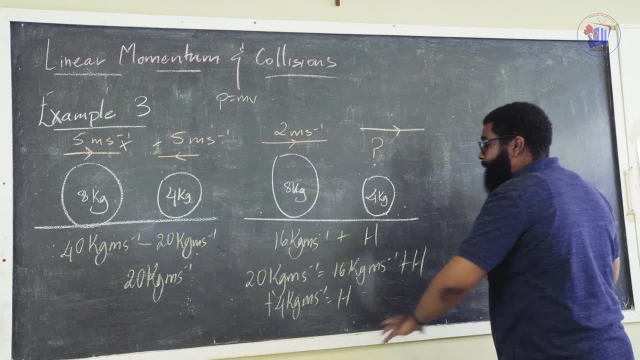 numbers that give us these values, numbers that give us these values: um. so the velocity of the four um. so the velocity of the four um. so the velocity of the four kilogram mass, kilogram mass, kilogram mass. from this equation, the velocity of this. from this equation, the velocity of this. 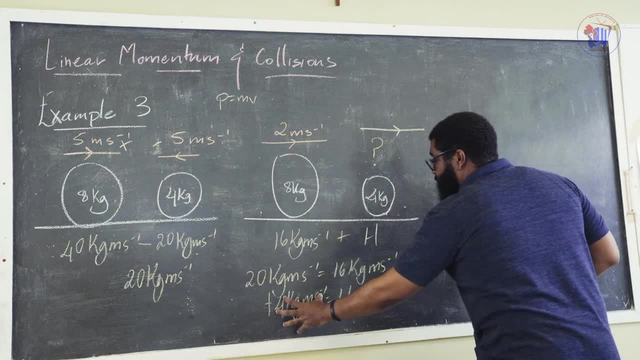 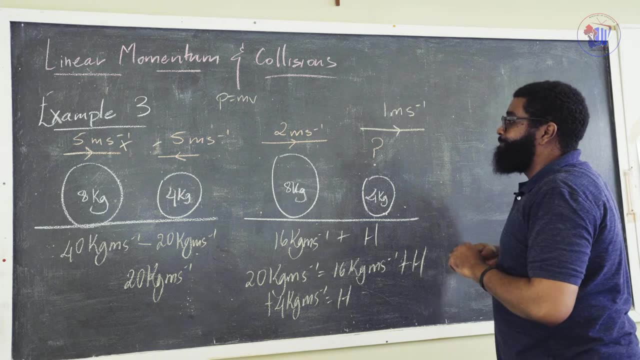 from this equation. the velocity of this would be the momentum divided by the. would be the momentum divided by the. would be the momentum divided by the mass mass. mass. four divided by four gives us one. four divided by four gives us one. four divided by four gives us one meter per second in that direction. 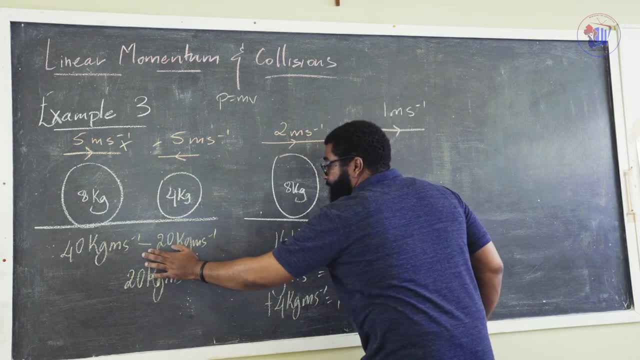 meter per second in that direction. meter per second in that direction. so opposite directions, we subtract. so opposite directions, we subtract. so opposite directions, we subtract. and over here and over here and over here, we add this to the unknown, equate it to. we add this to the unknown, equate it to. 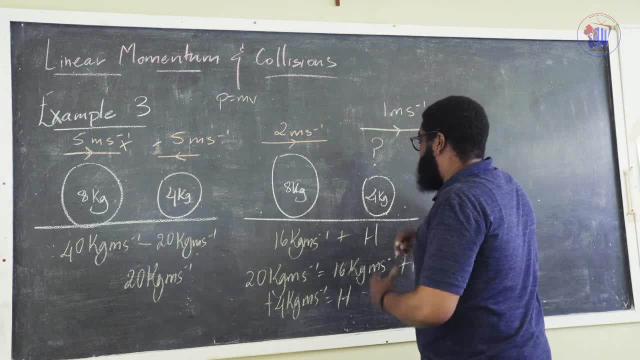 we add this to the unknown, equate it to what we got there, what we got there, what we got there. we do our algebra. our momentum is four. we do our algebra. our momentum is four. we do our algebra. our momentum is four kilogram meters per second. 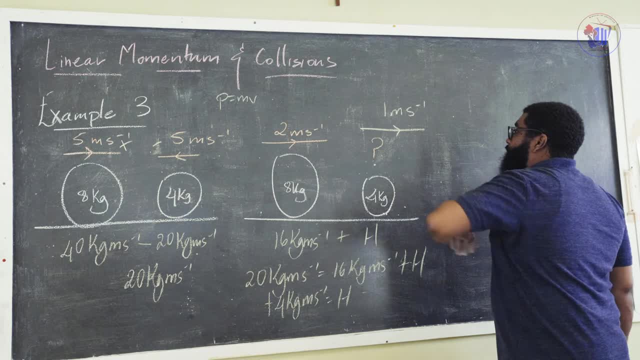 kilogram meters per second. kilogram meters per second in that direction. therefore, our velocity in that direction, therefore, our velocity in that direction, therefore our velocity is one meter per second, is one meter per second, is one meter per second in that direction. this is our third example. 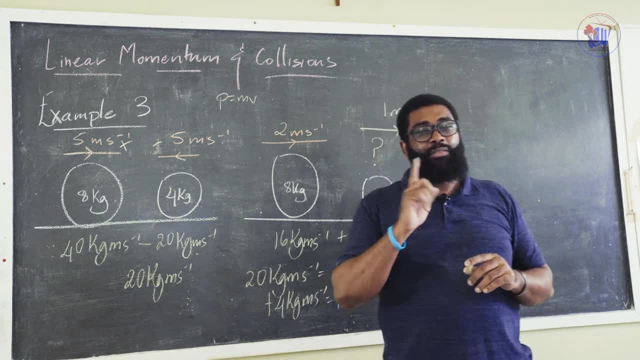 in that direction. this is our third example in that direction. this is our third example. now we have. now we have. now we have one more example to look at, one more, one more example to look at one more, one more example, to look at one more example, and i'll change my chalk. 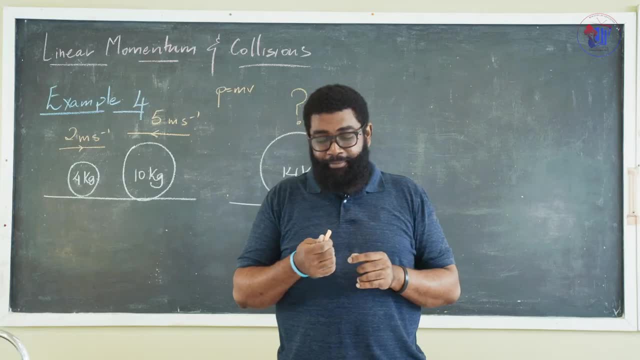 example and i'll change my chalk. example and i'll change my chalk. write my example on the board. i'll be write my example on the board. i'll be write my example on the board. i'll be right back, right back, right back. chalk changed. example on board changed. 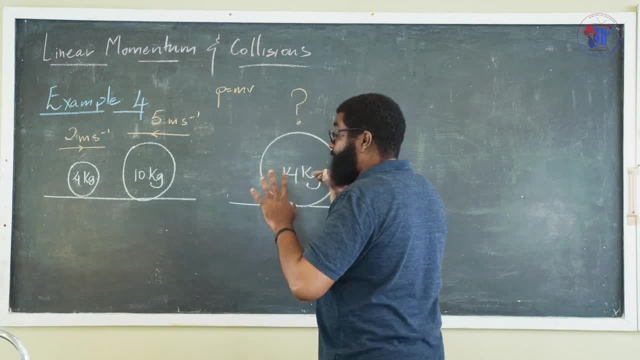 chalk changed. example on board changed. chalk changed. example on board changed. let's go. so here we have an interesting, let's go. so here we have an interesting, let's go. so here we have an interesting scenario, a possible scenario, scenario. a possible scenario, scenario, a possible scenario. okay, we have two objects of different. 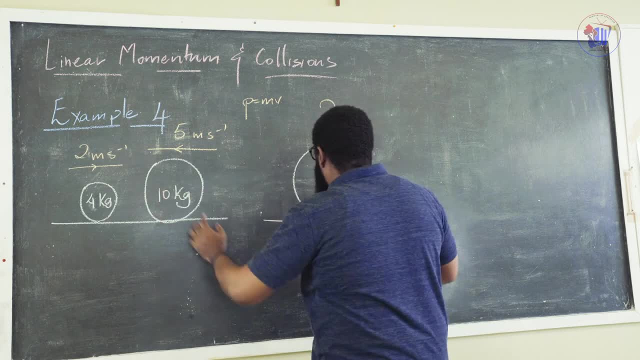 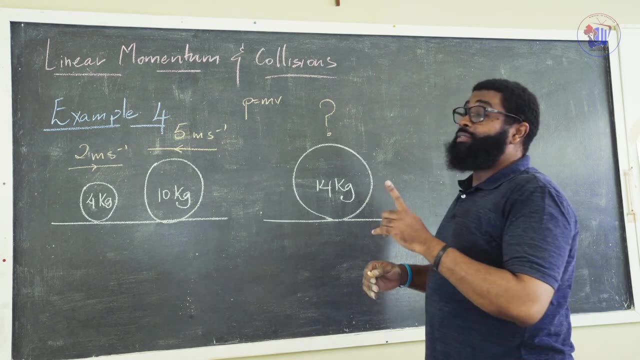 okay, we have two objects of different. okay, we have two objects of different masses traveling masses traveling masses traveling in opposite directions, that collide in opposite directions, that collide in opposite directions. that collide and then form one massive object, okay, and then form one massive object. okay, and then form one massive object- okay, this can happen as well. now, please note. 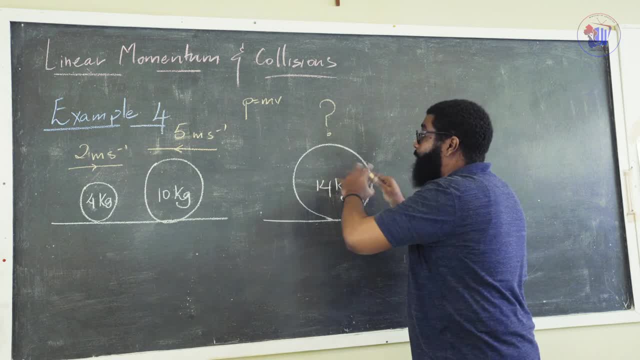 this can happen as well now, please note, this can happen as well now, please note, outside of this happening, you could, outside of this happening, you could, outside of this happening, you could actually have the opposite, actually have the opposite, actually have the opposite. you could have one object, one object for. 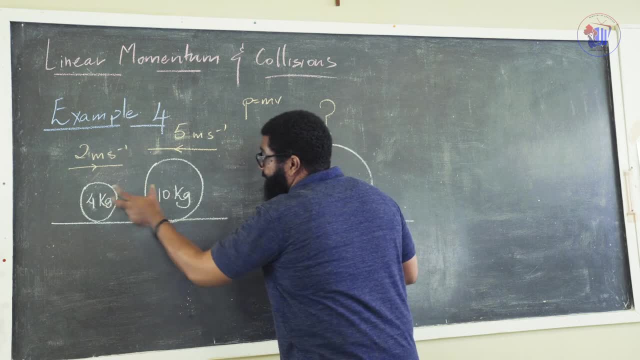 you could have one object, one object, for you could have one object, one object, for example, like example, like example, like exploding and creating multiple objects, exploding and creating multiple objects, exploding and creating multiple objects. so the reverse can happen, two can become. so the reverse can happen, two can become. 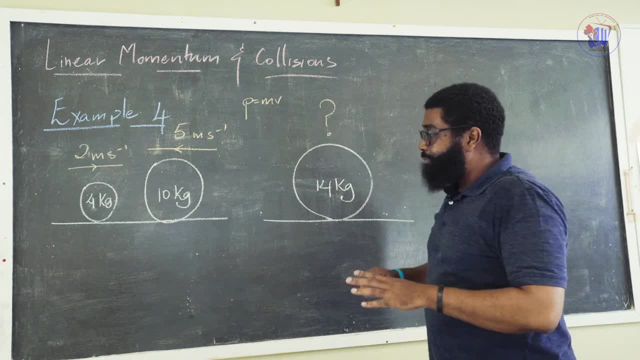 so the reverse can happen: two can become one and one, and one and one can become two or more now. one can become two or more now. one can become two or more now, using the ever faithful formula, and using the ever faithful formula, and using the ever faithful formula and assuming the collision to be totally, 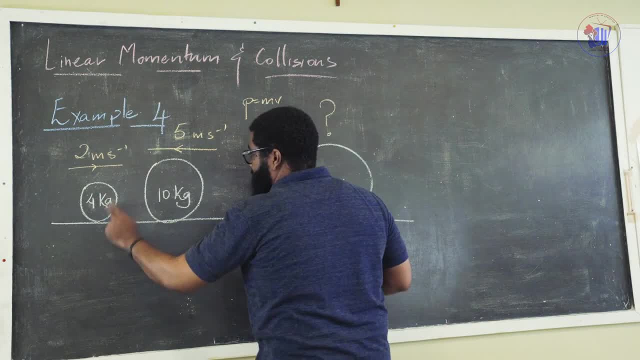 assuming the collision to be totally, assuming the collision to be totally elastic, elastic. elastic momentum is mass by velocity four by two. momentum is mass by velocity four by two. momentum is mass by velocity four by two. gives us, gives us, gives us eight. what a horrible eight. eight, what a horrible eight. 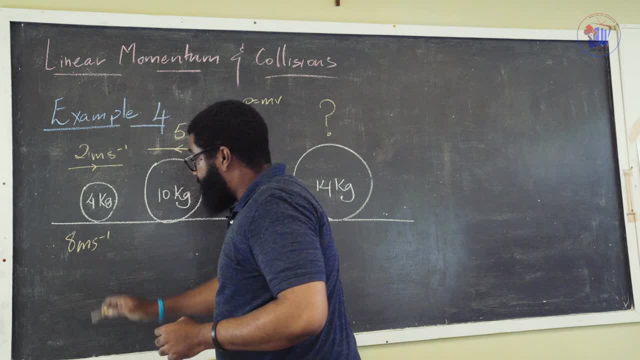 eight, what a horrible eight. eight meters per second. eight meters per second. eight meters per second. look at me, sinning father, forgive me. look at me, sinning father, forgive me. look at me, sinning father, forgive me. supposed to be kilogram meters per. supposed to be kilogram meters per. 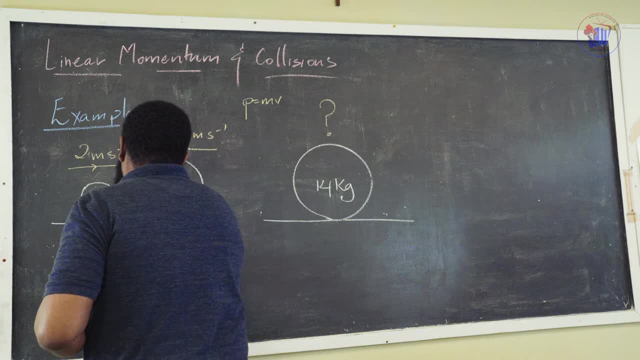 supposed to be kilogram meters per second. second, second: oh well, we all make mistakes, children. oh well, we all make mistakes, children. oh well, we all make mistakes, children. don't be ashamed to make yours, so four. don't be ashamed to make yours, so four. don't be ashamed to make yours. so four, twos, eight: kilogram meters per second. 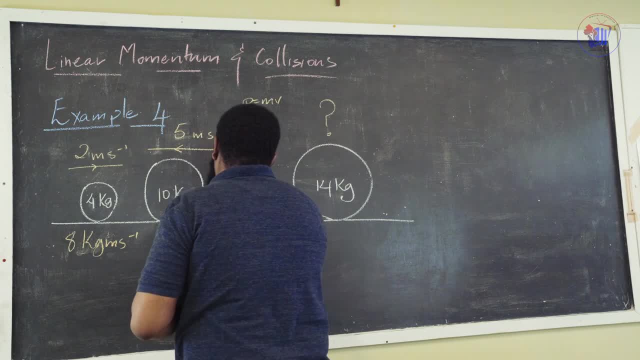 twos eight kilogram meters per second. twos eight kilogram meters per second, and ten by five is fifty, and ten by five is fifty and ten by five is fifty. kilogram meters per second. kilogram meters per second. kilogram meters per second. now, now. 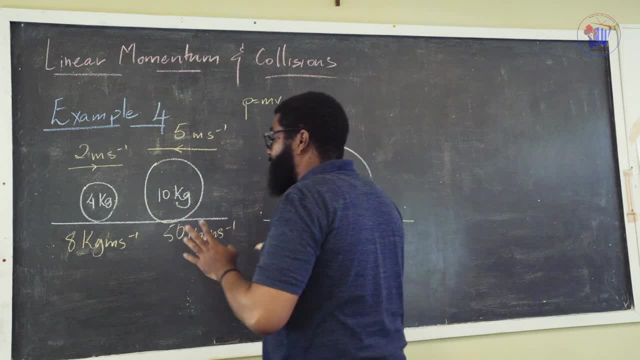 now they're traveling in opposite. they're traveling in opposite. they're traveling in opposite directions, directions, directions. okay. if i take this as positive, all okay. if i take this as positive, all okay. if i take this as positive, all right, right, right. if i take this this: 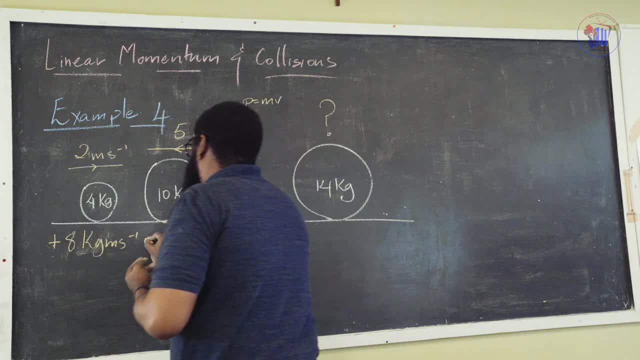 if i take this, this, if i take this, this, this is positive, is positive, is positive, going right is positive, going right is positive, going right is positive, and i take this is negative and i take this is negative and i take this is negative. i will end up with: 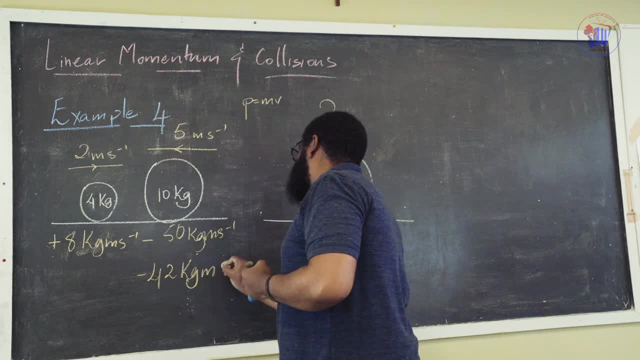 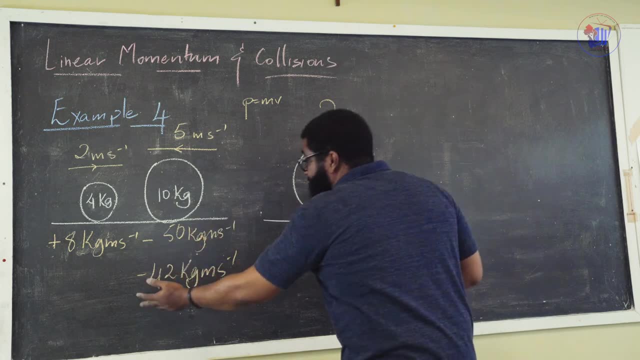 i will end up with. i will end up with: okay, yes, you can have a negative value. okay, yes, you can have a negative value. okay, yes, you can have a negative value. don't be scared of it. don't be scared of it. don't be scared of it. so i have no clue as to what happens with 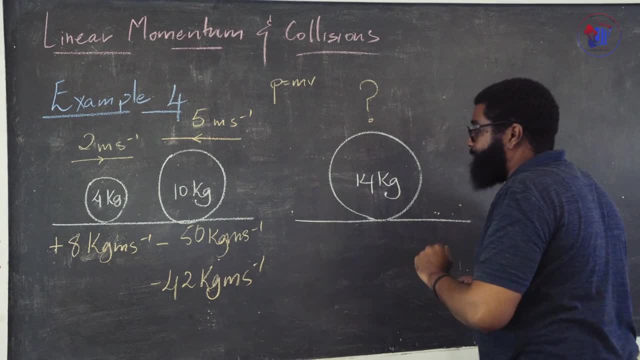 so i have no clue as to what happens with. so i have no clue as to what happens with this. there's just this. there's just this. there's just one object now. now i put 14 there. one object now. now i put 14 there. one object now. now i put 14 there because 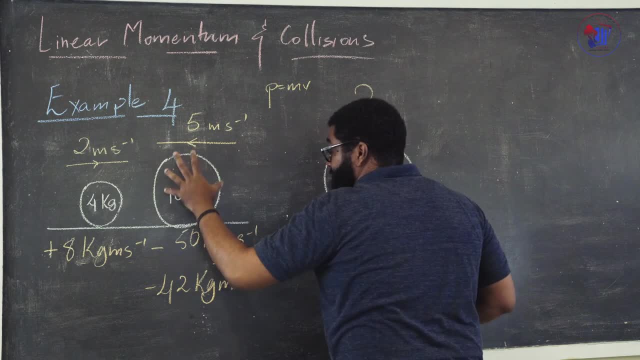 because, because i kind of give away what happens if i kind of give away what happens, if i kind of give away what happens if these two objects four, these two objects four, these two objects four kilograms and ten kilograms, if these kilograms and ten kilograms, if these kilograms and ten kilograms, if these two combine. 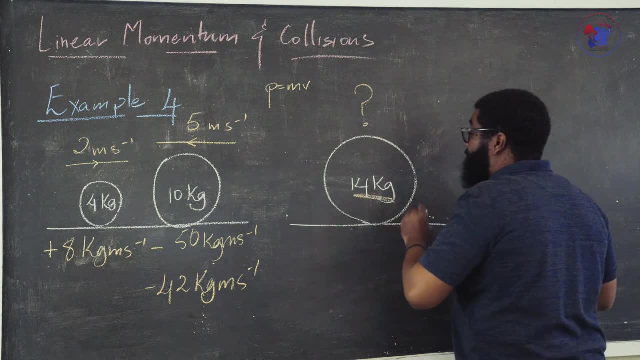 two combine. two combine: without losing any mass, the new mass of, without losing any mass, the new mass of, without losing any mass, the new mass of the object, the object, the object, the single object is now 14 kilograms. the single object is now 14 kilograms. the single object is now 14 kilograms. okay, that's the first thing. the second: 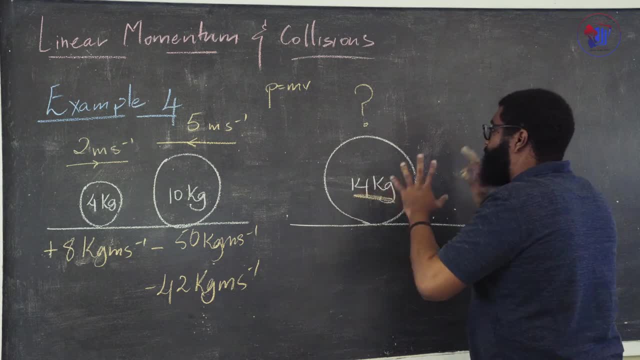 okay, that's the first thing. the second: okay, that's the first thing. the second thing, thing thing is that, because there's only one object, is that because there's only one object, is that because there's only one object, we don't know what and we don't know. 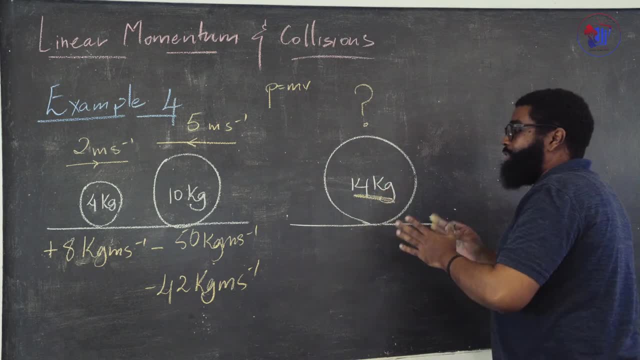 we don't know what and we don't know, we don't know what and we don't know what happens here. what happens here? what happens here? we have to depend on the principle of, we have to depend on the principle of, we have to depend on the principle of conservation of linear momentum. 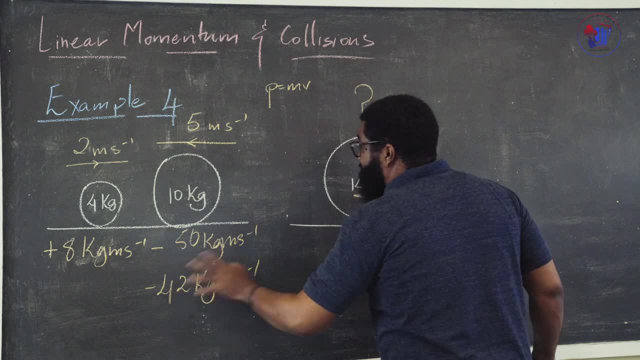 conservation of linear momentum. conservation of linear momentum. to explain this, to explain this, to explain this now, this minus 42 kilogram meters per now. this minus 42 kilogram meters per now. this minus 42 kilogram meters per second. second: second is essentially the momentum of this: 14. 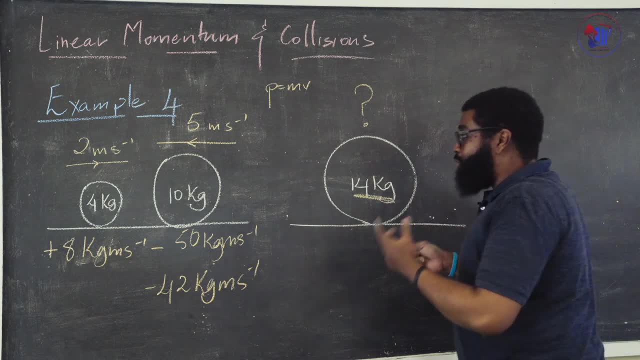 is essentially the momentum of this. 14 is essentially the momentum of this. 14 kilogram object. kilogram object. kilogram object. after the collision. so what it means is after the collision. so what it means is after the collision. so what it means is that this 14 kilogram meter. 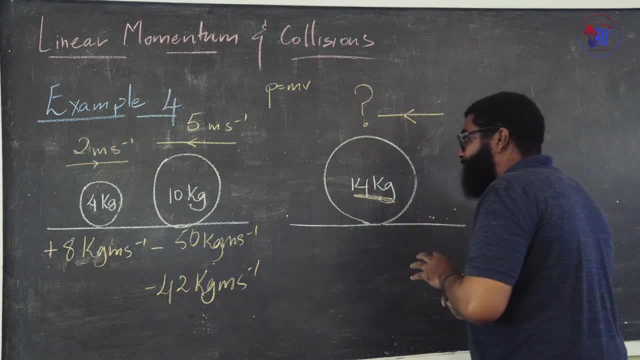 that this 14 kilogram meter, that this 14 kilogram meter, 14 kilogram object. sorry is moving to 14 kilogram object. sorry is moving to 14 kilogram object. sorry is moving to the left, the left, the left, like beyonce said um, and we just have. 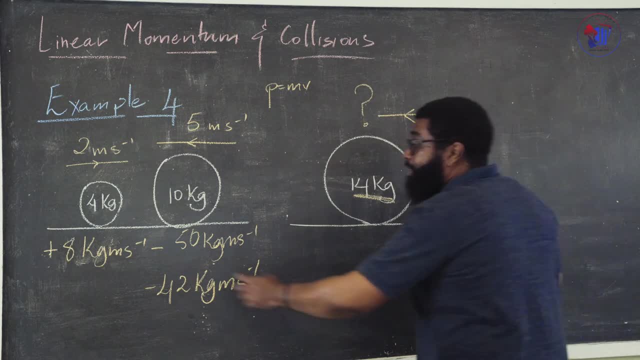 like beyonce said um, and we just have, like beyonce said um, and we just have to work out its velocity, to work out its velocity, to work out its velocity. why is it going to the left? because we. why is it going to the left? because we. 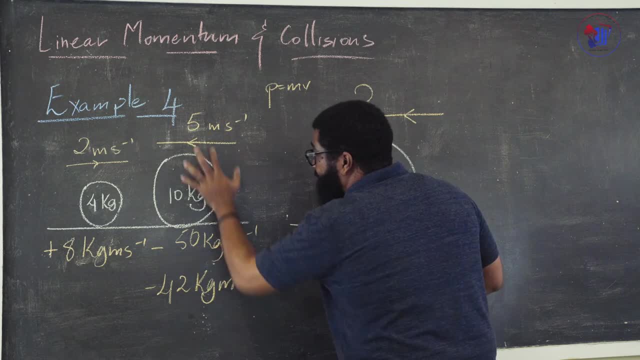 why is it going to the left? because we took, took, took this, this value here, this, this value here, this, this value here as negative. that's why we have a as negative, that's why we have a as negative, that's why we have a negative momentum here. 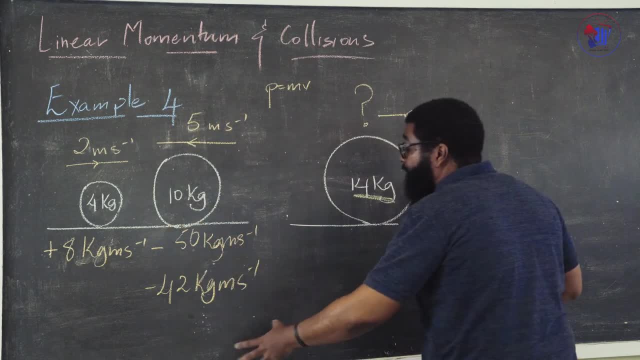 negative momentum here, negative momentum here. this direction is negative. this momentum, this direction is negative. this momentum, this direction is negative. this momentum is negative, is negative, is negative. the total momentum is negative. therefore, the total momentum is negative. therefore, the total momentum is negative. therefore, this moves in the negative direction. 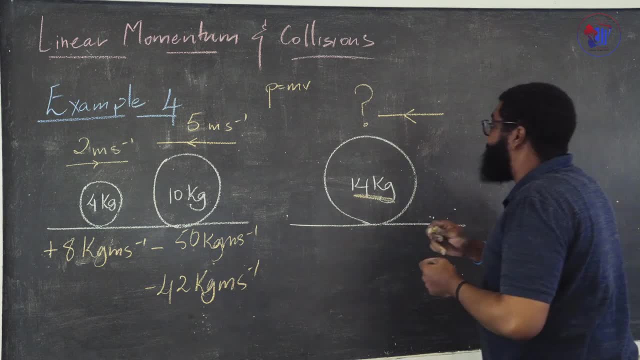 this moves in the negative direction. this moves in the negative direction which, for the sake of this example, is which, for the sake of this example, is which, for the sake of this example, is to the left, to the left, to the left, anyways, again applying the formula that, 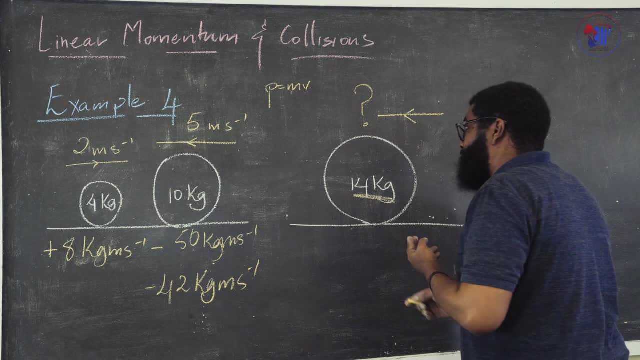 anyways again applying the formula that, anyways again applying the formula that momentum is mass times velocity. momentum is mass times velocity. momentum is mass times velocity. to find the velocity we divide momentum. to find the velocity we divide momentum. to find the velocity we divide momentum minus four to two, not just four to two. 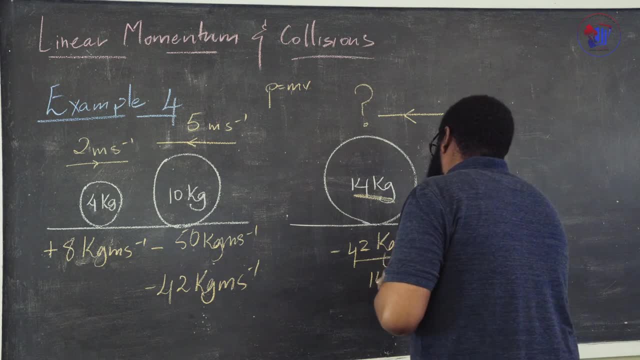 minus four to two, not just four to two. minus four to two, not just four to two. kilogram meters per second kilogram meters per second kilogram meters per second by by by 14, 3, 10, 30, 3, 4, 12, 14, 3, 10, 30, 3, 4, 12. 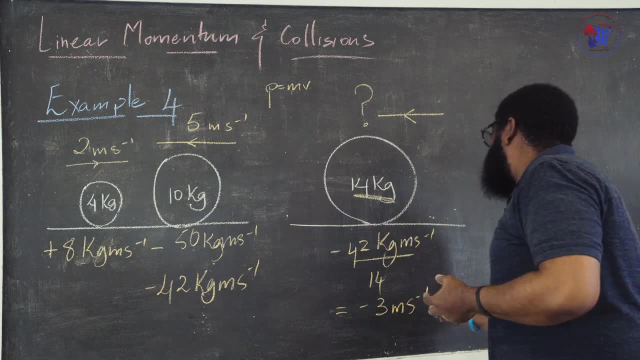 14, 3, 10, 30, 3, 4, 12. i do believe, if my math is correct, this: i do believe, if my math is correct, this: i do believe, if my math is correct, this is three meters per second. is three meters per second. 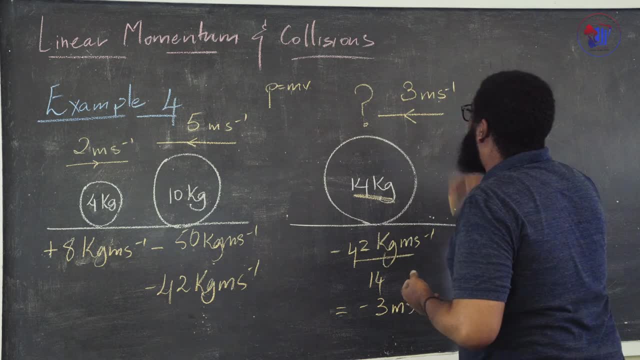 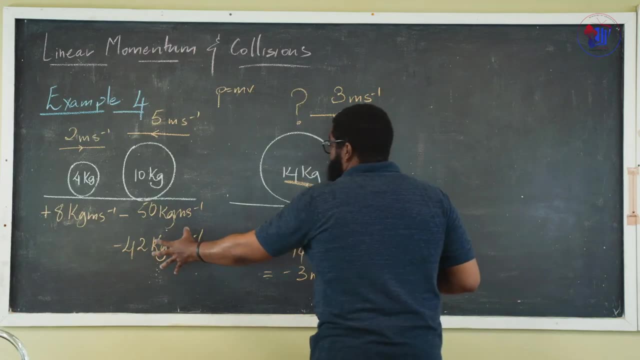 is three meters per second. so our object, our new object, so our object, our new object, so our object, our new object moves to the left at three moves to the left at three moves to the left, at three meters. the second total momentum before they collide is the. 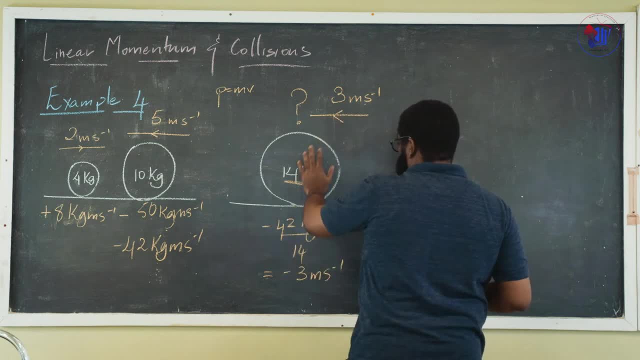 total momentum before they collide is the total momentum before they collide is the same as the total momentum after, same as the total momentum after, same as the total momentum after. so that gives us our 42 over here. so that gives us our 42 over here. so that gives us our 42 over here. dividing by 14 gives us our 3, which is: 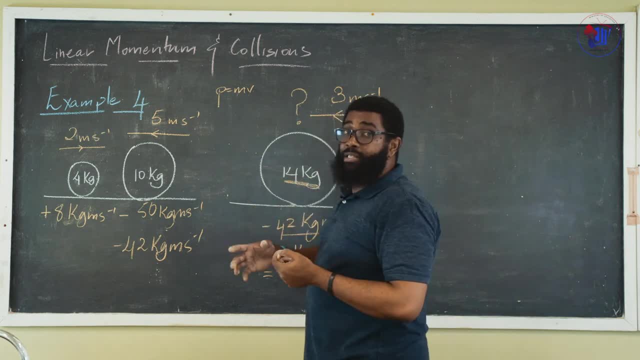 dividing by 14 gives us our 3, which is dividing by 14 gives us our 3, which is our velocity, our velocity, our velocity. these are four of the most common. these are four of the most common. these are four of the most common examples that you're going to find. 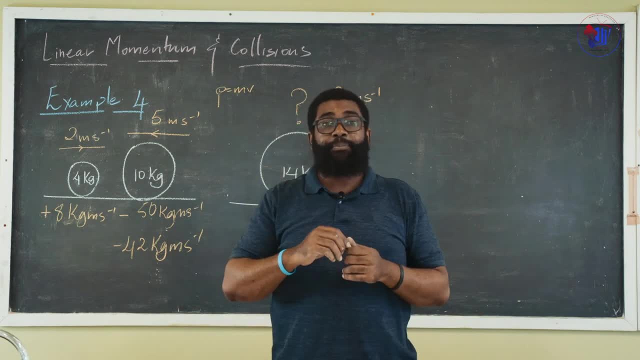 examples that you're going to find, examples that you're going to find: okay, these are the four now the cool. okay, these are the four now the cool. okay, these are the four now. the cool thing is you just have to remember that thing is. you just have to remember that. 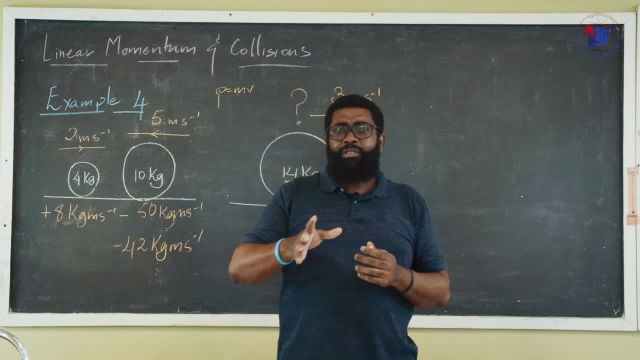 thing is, you just have to remember that you apply the principle of conservation, you apply the principle of conservation, you apply the principle of conservation of linear momentum. you don't need to do of linear momentum, you don't need to do of linear momentum, you don't need to do anything fancy: mass by velocity for each. 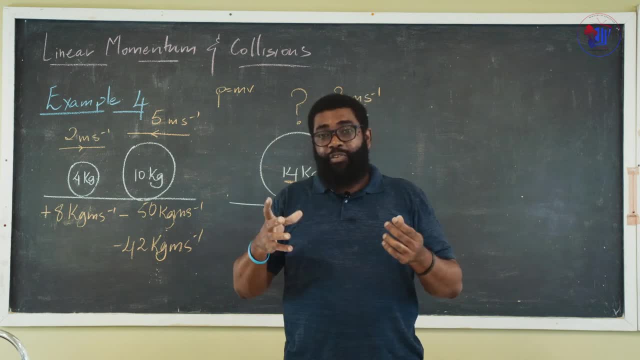 anything fancy: mass by velocity for each. anything fancy: mass by velocity for each object, with direction taken into object. with direction taken into object, with direction taken into consideration. you find your total. you consideration. you find your total. you consideration. you find your total. you equate it to either: before they collide: 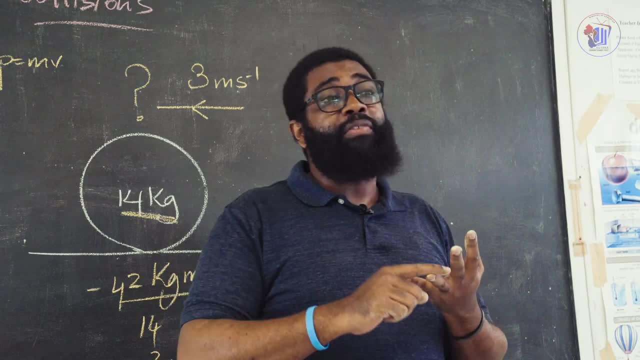 equate it to: either before they collide. equate it to: either before they collide or after they collide. you find your or after they collide. you find your or after they collide. you find your unknown momentum. you divide by mass to unknown momentum. you divide by mass to: 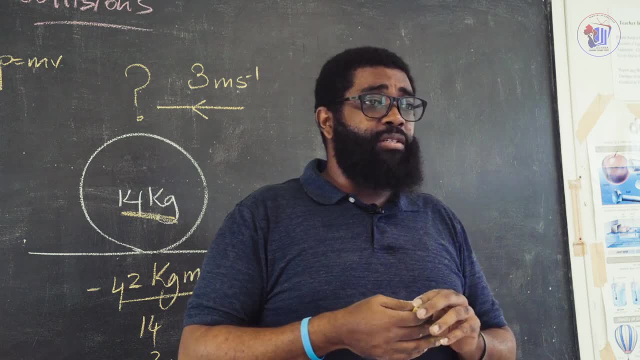 unknown momentum. you divide by mass to find your unknown velocity. find your unknown velocity, find your unknown velocity. that's what you do in most cases, that's what you do in most cases, that's what you do in most cases. so to quickly recap today's lesson. so to quickly recap today's lesson, 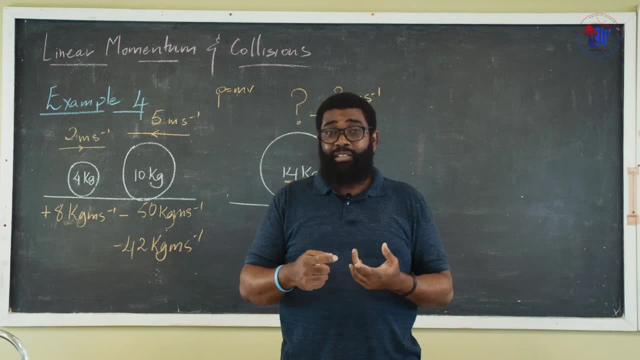 so to quickly recap today's lesson: inelastic collisions are collisions in. inelastic collisions are collisions in. inelastic collisions are collisions in which kinetic energy is not conserved. which kinetic energy is not conserved. which kinetic energy is not conserved. elastic collisions are collisions in. 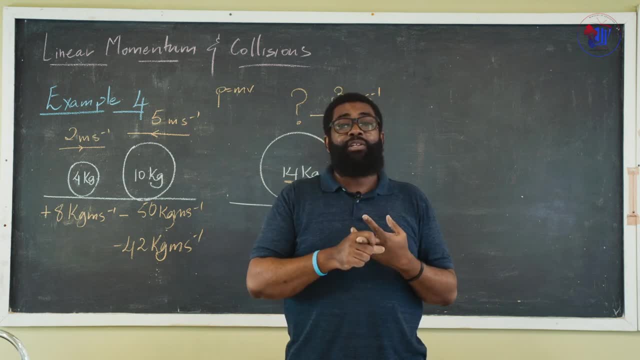 elastic collisions are collisions in. elastic collisions are collisions in which kinetic energy is conserved and which kinetic energy is conserved and which kinetic energy is conserved. and the principle of conservation of linear, the principle of conservation of linear, the principle of conservation of linear momentum states that the vector sum of 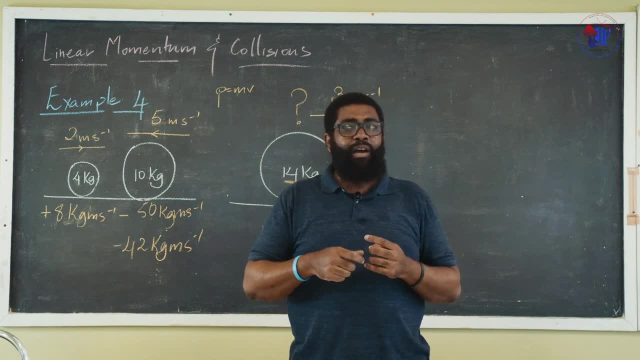 momentum states that the vector sum of momentum states that the vector sum of momentum before a collision is equal to momentum before a collision. is equal to momentum before a collision. is equal to the vector sum of momentum. the vector sum of momentum, the vector sum of momentum after a collision, provided that kinetic 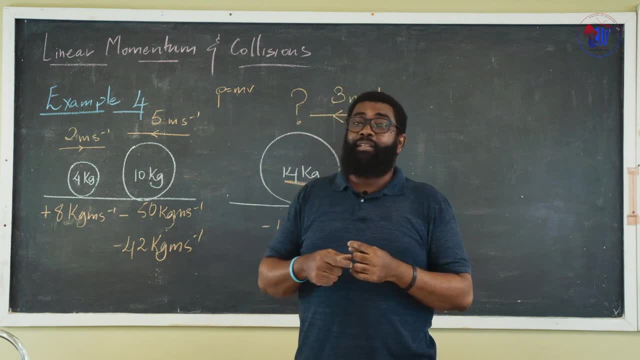 after a collision, provided that kinetic after a collision, provided that kinetic energy is conserved, energy is conserved, energy is conserved. this is what we apply today. this is what this is what we apply today. this is what this is what we apply today. this is what i hope you learned today. 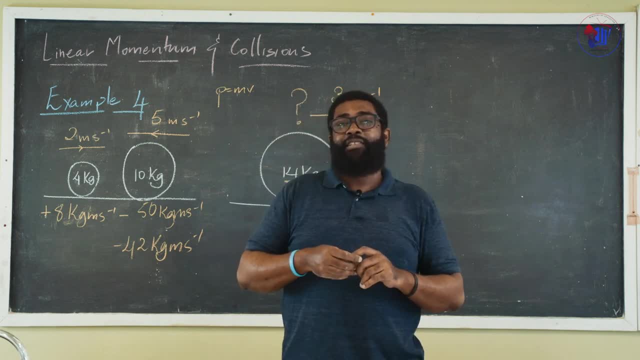 i hope you learned today. i hope you learned today and i will see you next time, on the next, and i will see you next time on the next, and i will see you next time on the next episode of csec physics with me. episode of csec physics with me.